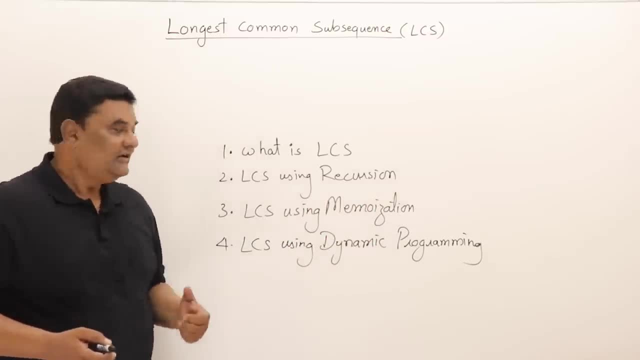 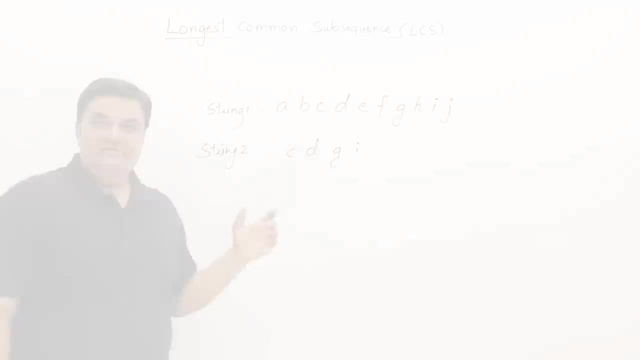 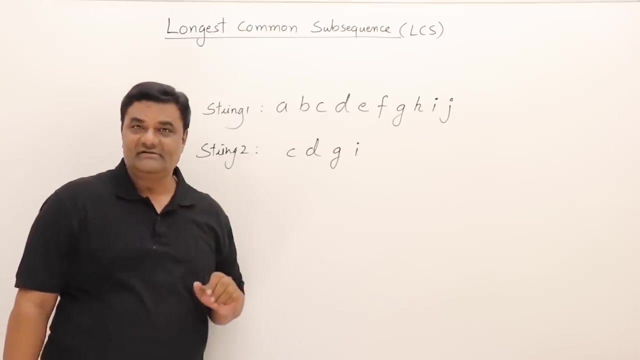 here I will also show you LCS using memoization. Then, finally, we will solve LCS using dynamic programming. So let us start with the problem. Let us understand the problem. See here there are two strings, So there is nothing like substrings here. See, in KMP algorithm we will have main string and 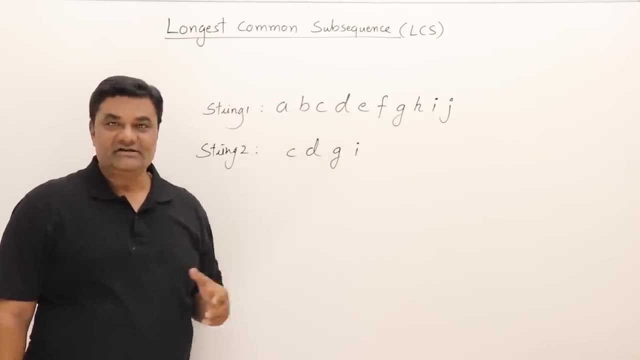 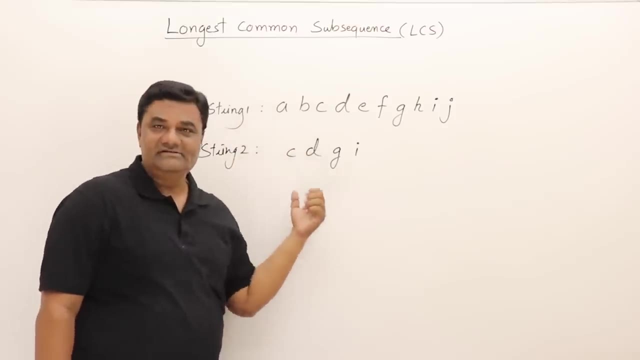 substring and the substring we will search in the main string. No, here we have two different strings. Here you can see that I have taken this as a longer size and this is a smaller size. This is not a substring at all. We are not. 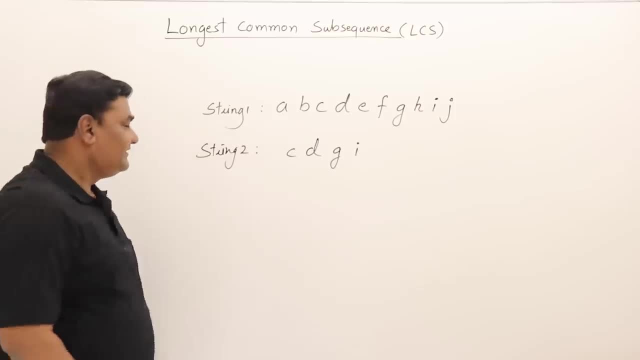 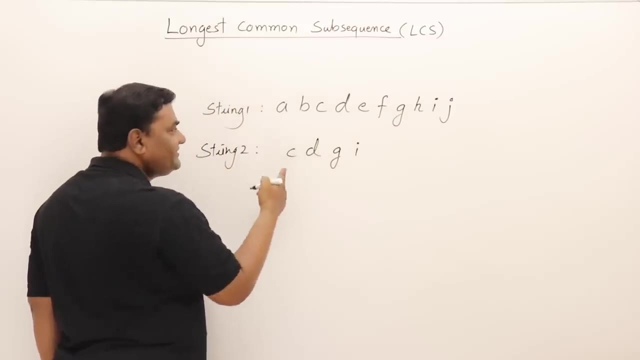 finding exact match. Now let us understand what it is See here. there are some set of characters, and the same characters. they are appearing here also, and we want to find out which set of characters are coming in sequence. So let us start C from this one. I will check. 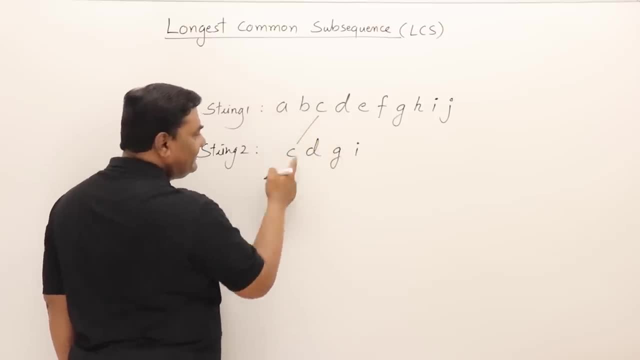 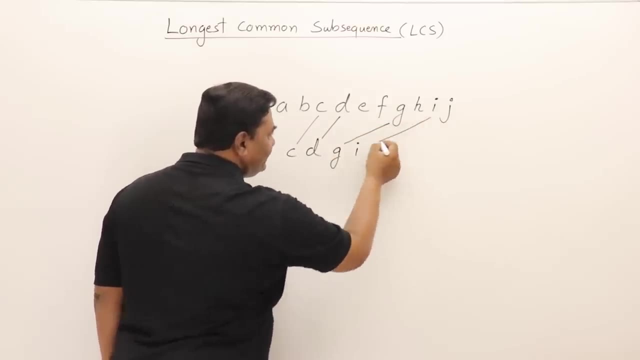 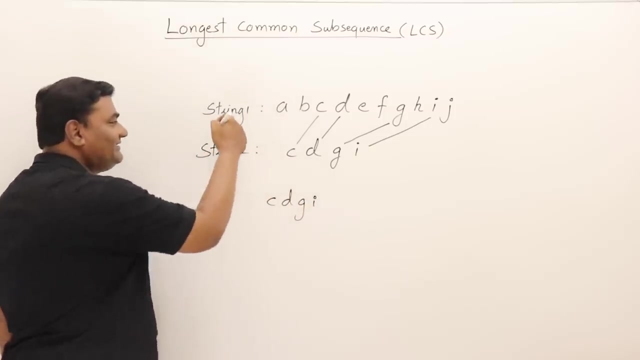 because this is smaller. C, yes, C is there. yes, D, yes, it is also matching with this one. G is matching with this one and I is matching with this one. Yes, this is a sequence: C, D, G, I is a sequence that is there in the string one. No doubt the characters are not together, but they. 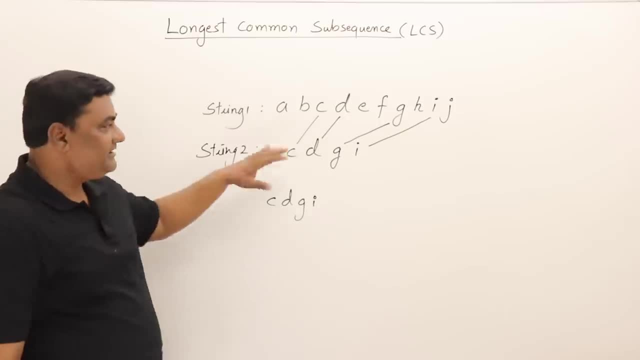 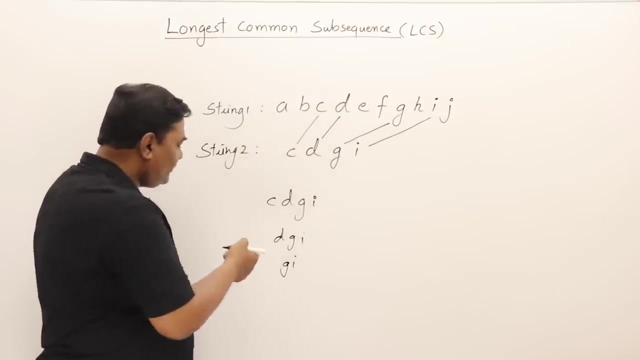 are coming in the same order. that is same sequence. they are appearing in another string, So this is the longest. This is common subsequence From this one. even I can say that D G I is appearing there, or I can say just G I is appearing there, but what is longest? C, D, G, I is longest. So this one example. 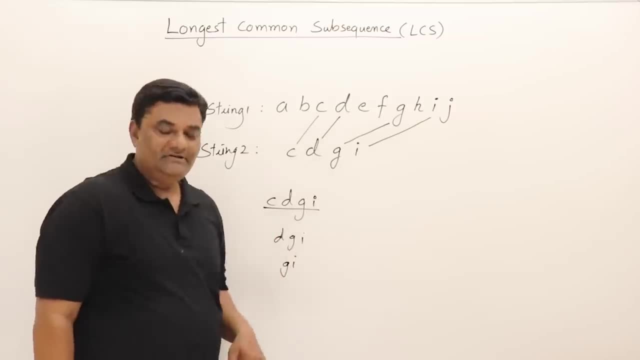 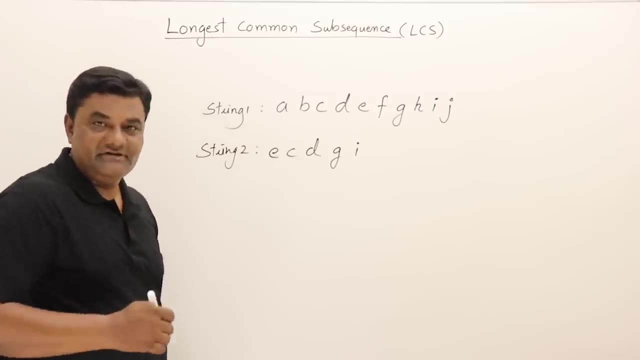 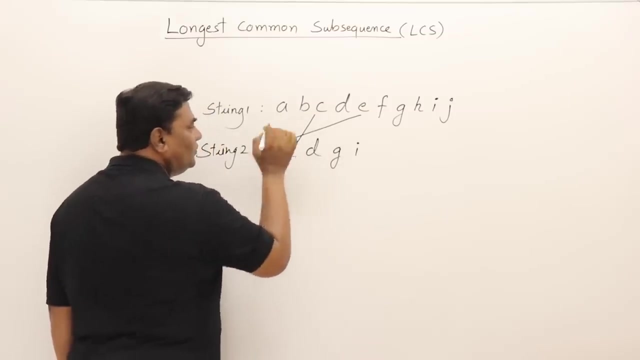 I will make some changes in this one. I will show you another example. In the same example, I will add A here. Now let us try to find out the subsequence in this one. E: this is matching. yes, it is matching with this one. C- yeah, it is matching. No, when you are finding the matches, you 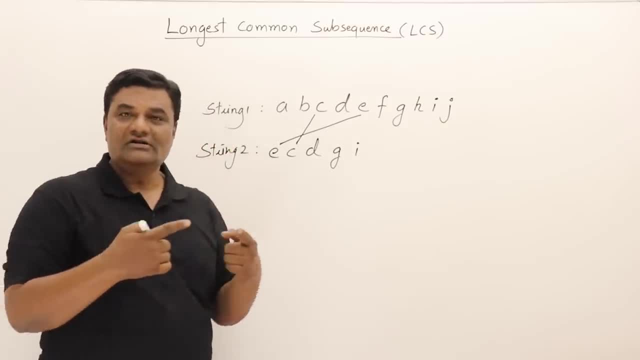 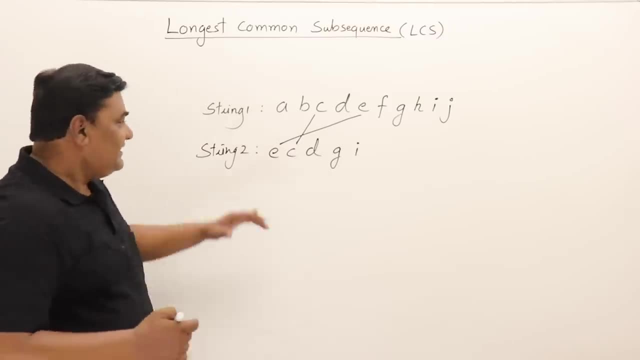 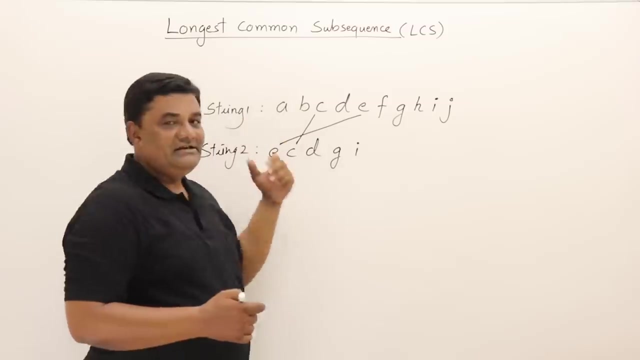 should take care that these matching should not intersect with each other. If you draw lines between them, they should not intersect with each other. So it means that E has appeared here. then C should be following that E, not at the back side of E, So you can take only those characters that. 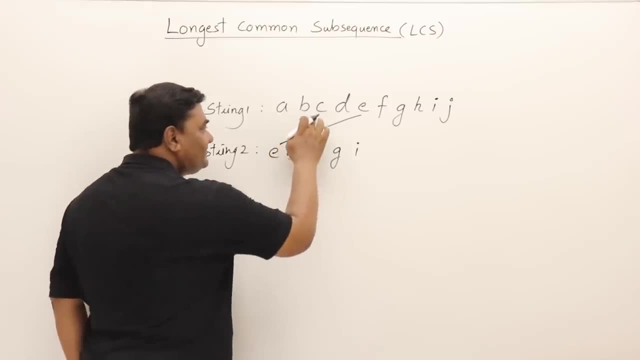 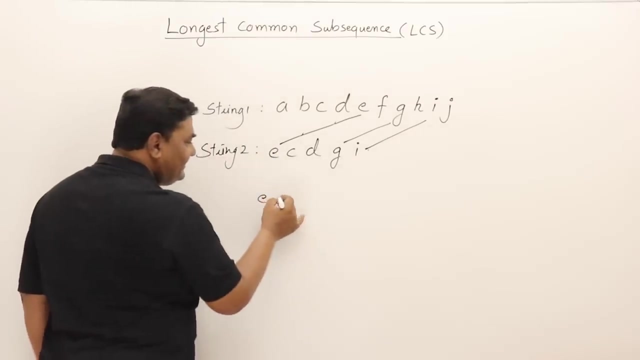 are coming after E, So C I should skip. Then. is there anything matching D? no, this is also intersecting, So this is coming before E. So then next is what G? yes, this is matching I. so one subsequence I got is E, G, I Is. 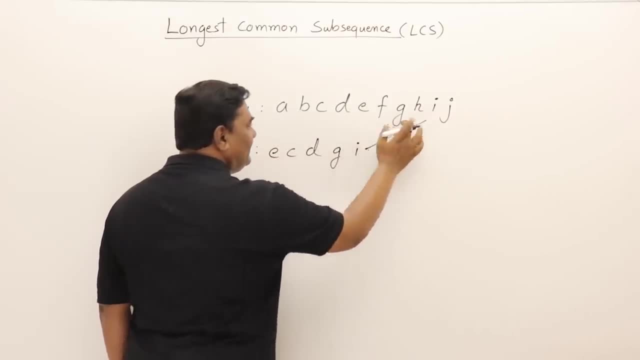 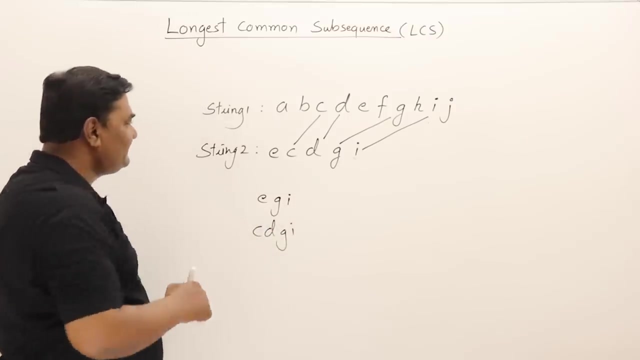 there any other subsequence? let me try. Instead of starting from E, I will start from C. yes, matching D. yes, matching G and I. yes, C, D, G, I is also there. So E, G, I is also a subsequence present there That is common in both the strings. 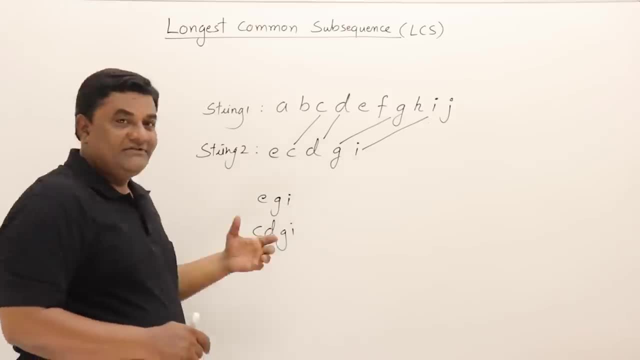 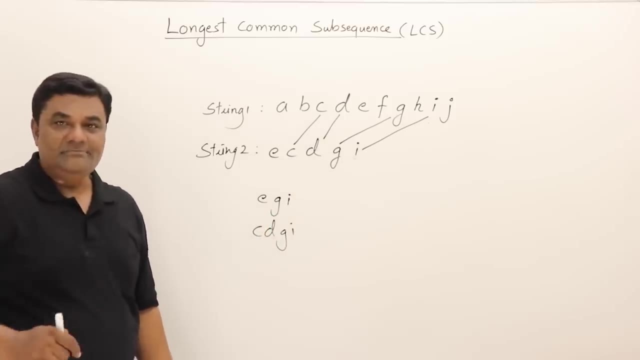 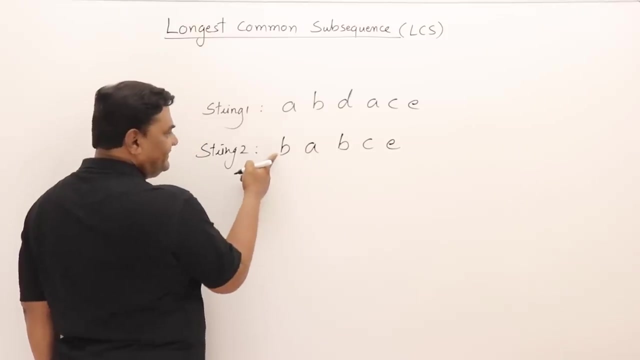 right and C D G I is also there. But which is the longest subsequence? C D G I is the longest subsequence. I will take one more example and show you One more example: two strings. let us find out what is the longest subsequence. Let us start with this one from second string and comparing. 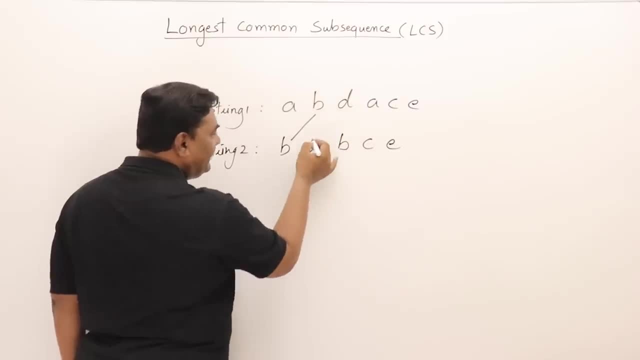 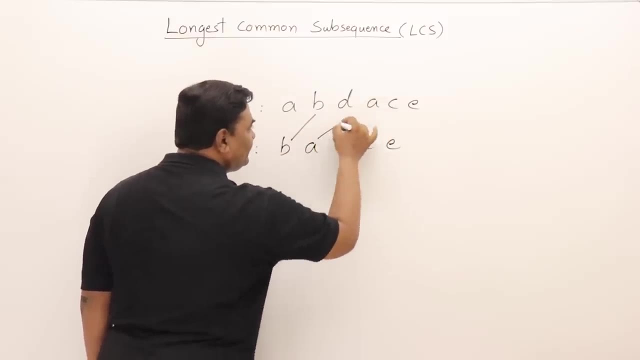 with the first string. A is found here. yes, A is found. no, you should not take the characters that are before the match. Then this A is also there here also, yes, it is there. Then B: then B is in this direction. no, there is. 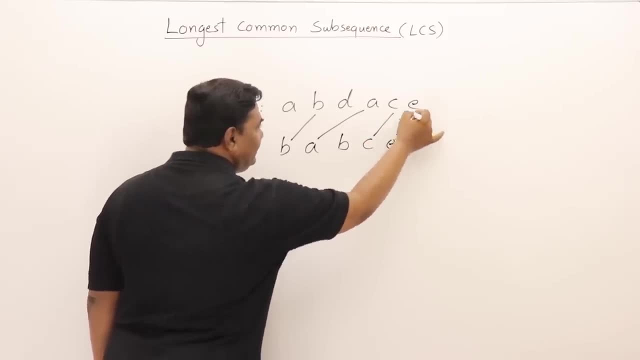 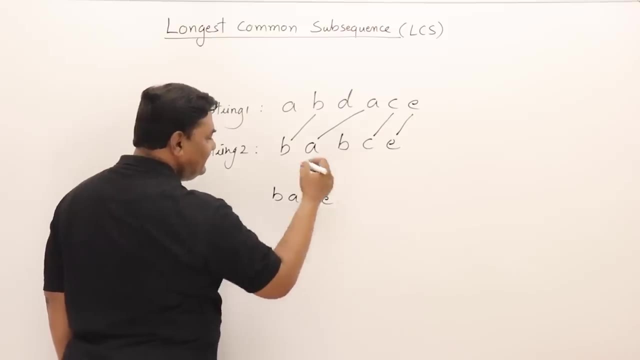 no B, followed by A. So C is there, yes, E is there. So what are the alphabets? I got B, A, C, E. this is one. Let us try. is there any other one? Next of B, I will start from A. So this A is matching here, yes, Then B is matching with this one. 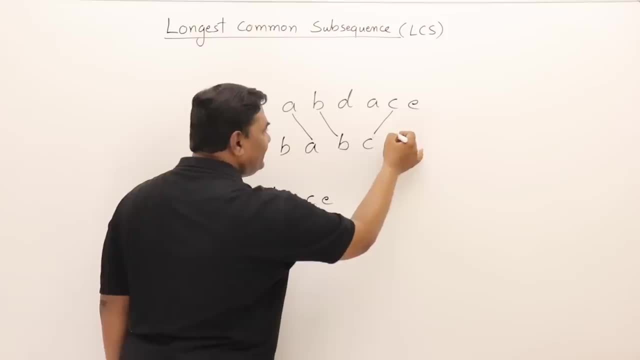 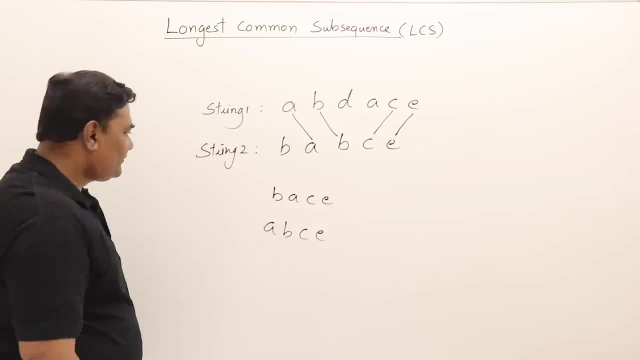 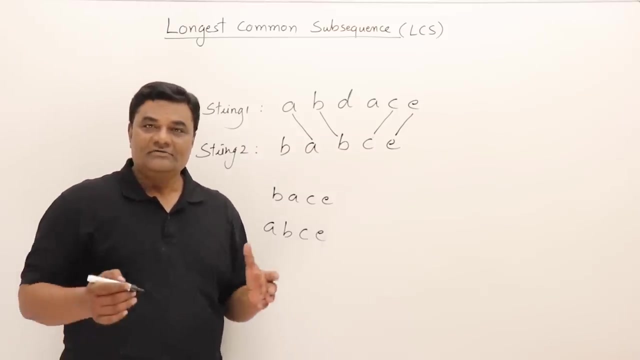 C is matching, it is not intersecting, Though the direction is different. E is there. So A, B, C, E. So we have two subsequences which are of same length. yes, There can be multiple subsequences with same length also. So that is it. The problem is finding whether the set of characters in these 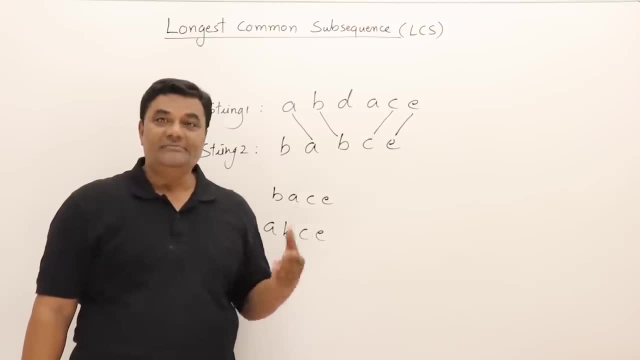 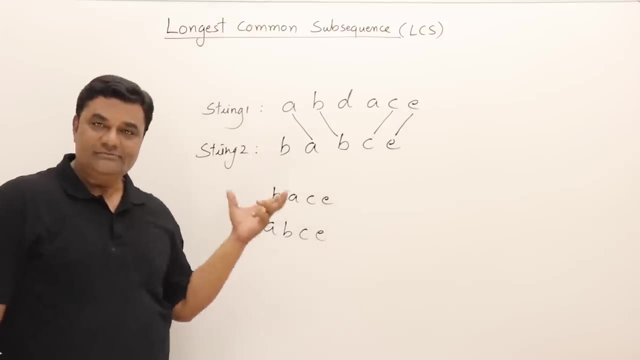 two strings are matching or not. The matching characters need not be continuous. Now let us see how we can solve it using recursion. So I will write an algorithm and I will take a very small problem and show you how recursion works on that. Then we will see memoization also. 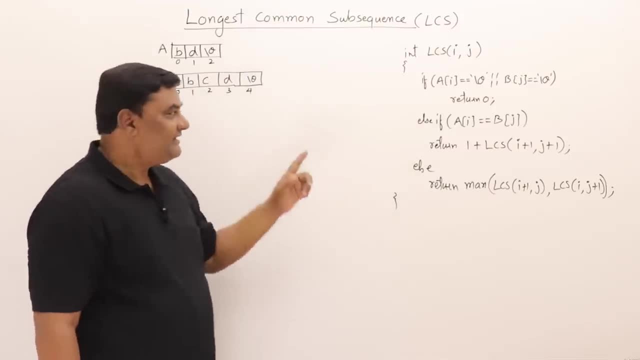 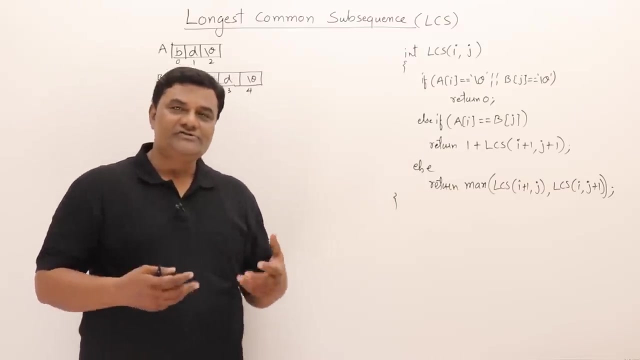 This is an algorithm for finding longest common subsequence and it is a recursive algorithm. I have taken a small size, two strings, and let us trace this algorithm and see how recursion works. I will draw recursion tree Then after that I will also show how memoization can make. 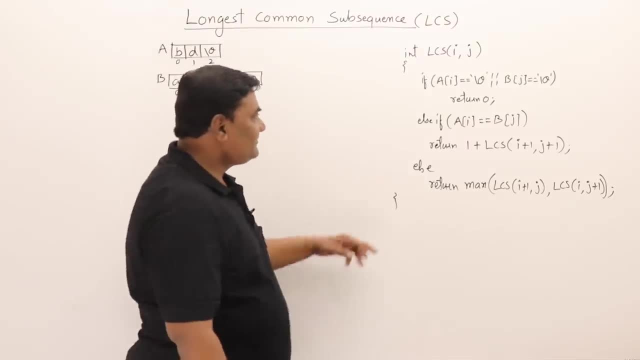 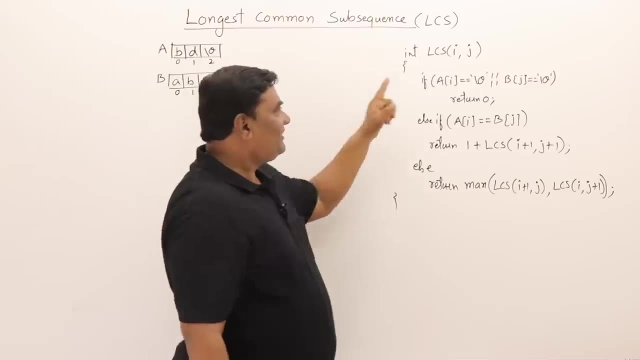 it faster. First of all, let us look at the algorithm. See. these are the strings, so they are terminated by slash zero and the indices are starting from zero onwards. Let us see what are the parameters of algorithm. See. it is taking i and j. that are the starting. 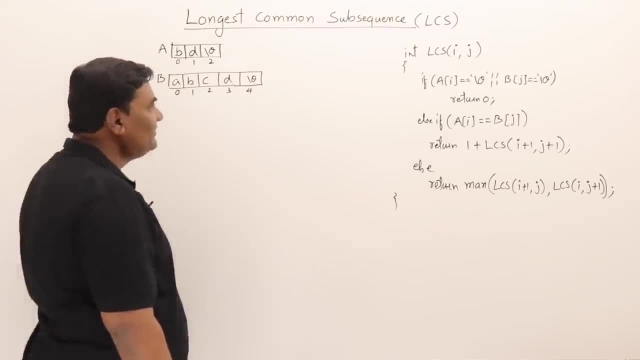 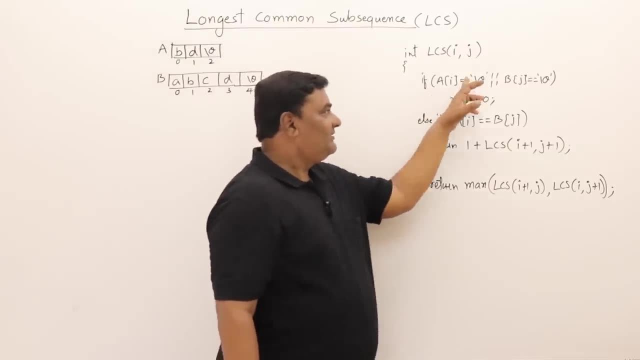 indices of A and B that initially they will be 0- 0.. So i and j will work as indices for two strings, A and B. Then if the alphabet is slash, zero, any one of them is 0, then return 0. If they match. 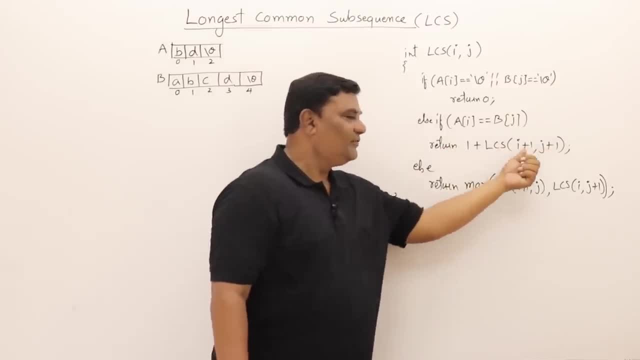 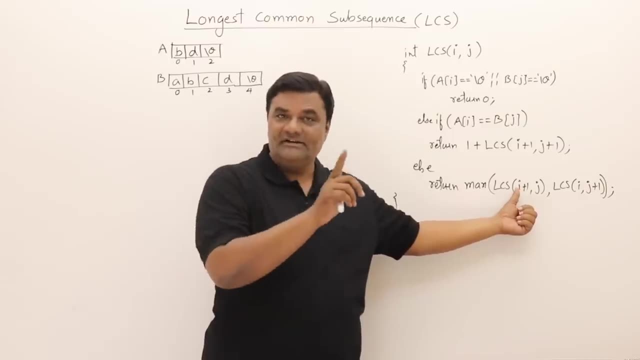 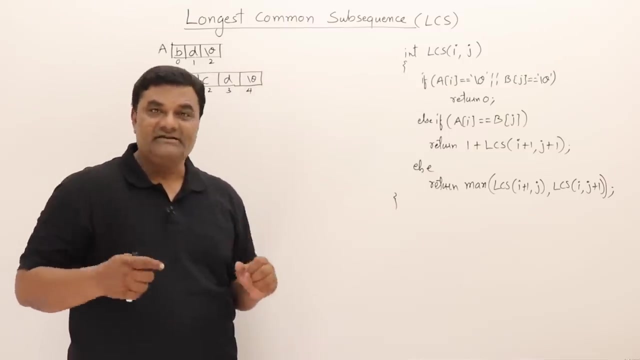 then add 1 and move to the next alphabet in both A and B. If there is no match, then check. either way, move one alphabet in first string A or move alphabet in second string B and check whichever is giving maximum. take that Most of the time this condition will be satisfied. 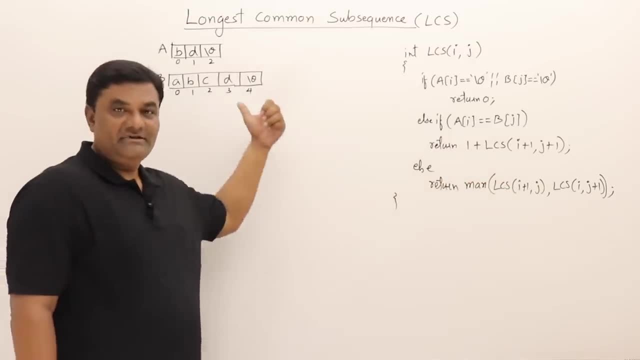 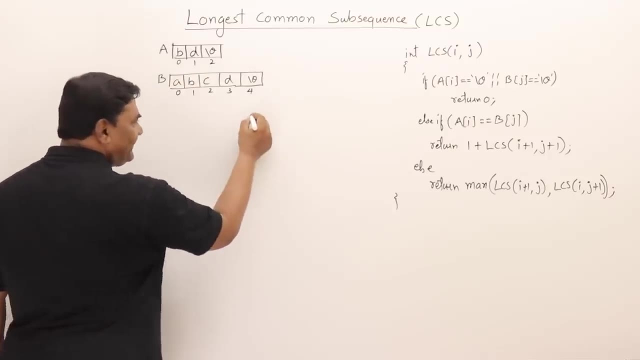 and let us see the tracing. Let us trace this. See, initially indices are 0: 0. so for tracing purpose I will write it like this: A of 0 and B of 0, and what are those alphabets B and A? so this is B and A. 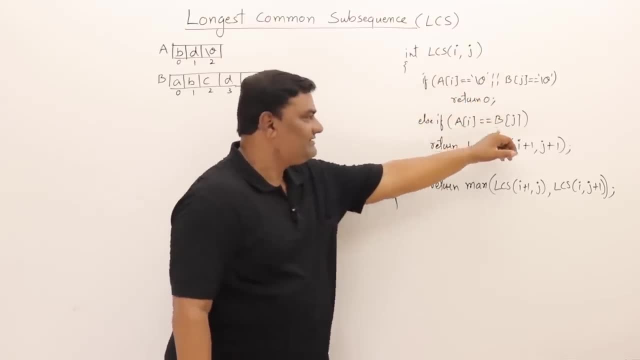 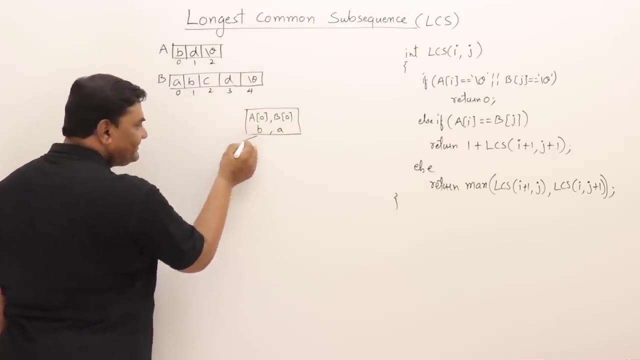 Let us check here. this condition is not true. and are they same? they are not same. enter into this part. So for this call, actually it will make two different calls again. This is one call where A will be moved to the next alphabet, that is, 1, and B remains 0 only. 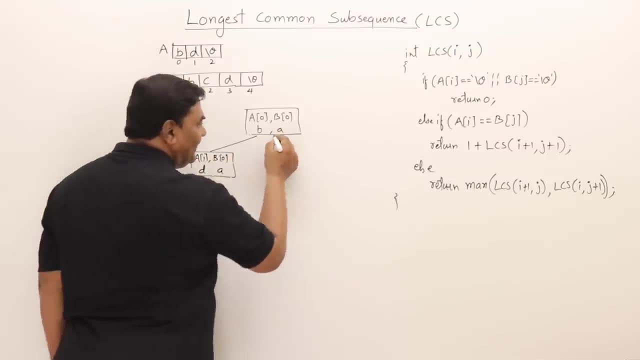 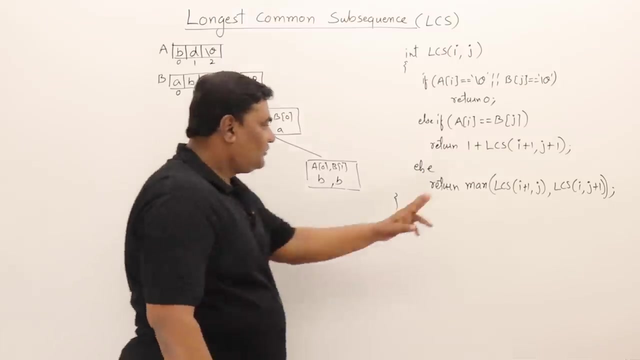 So what are those alphabets? D and this is A only Otherwise. one more is: A remains at 0, only comma B moves to the next alphabet. so A will be B and B of 1 is what B Two calls it will make out of these two calls. whichever is giving maximum, it will take that result. 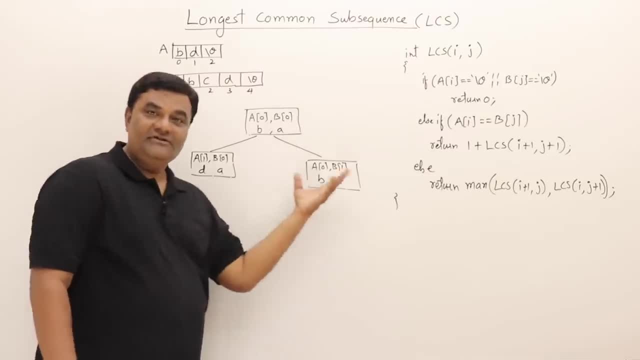 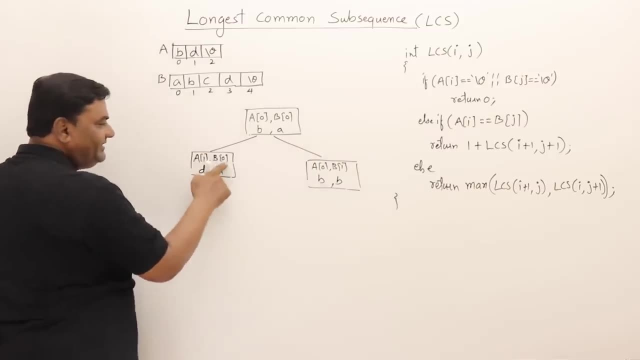 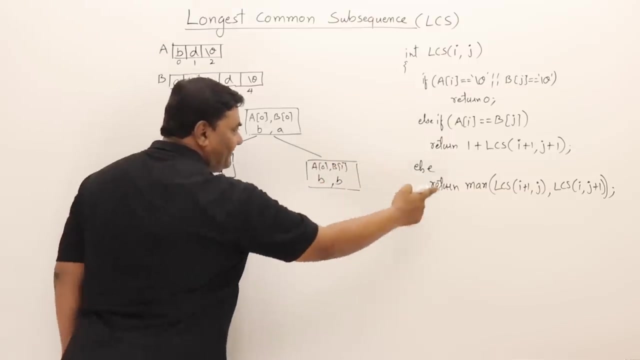 So for that, first this has to be completed, then afterwards this can be completed. So let us continue with this one. So for this again, a call is made where I is 1 and B, J is 0. So this first condition fails. they are not slash 0 and even they are not matching. 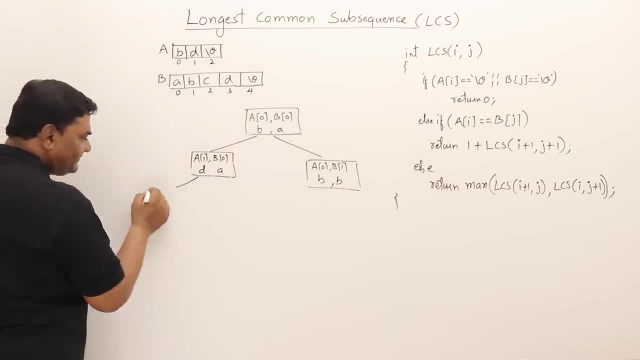 so again it enters into the third part. So two calls. so the first call is what? A will move to the next alphabet, from 1 it will go to 2 and the B remains 0 only. So what are these alphabets? A2 is what slash 0 and B0 is A only and this side again one. 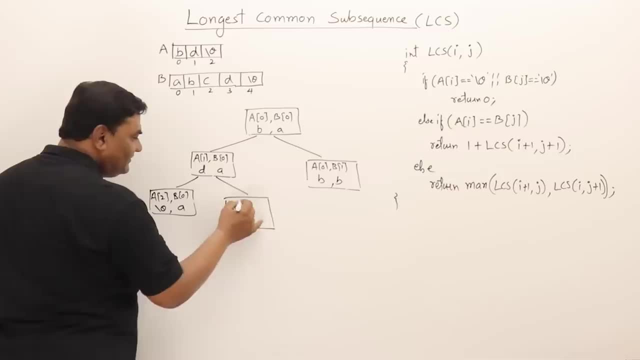 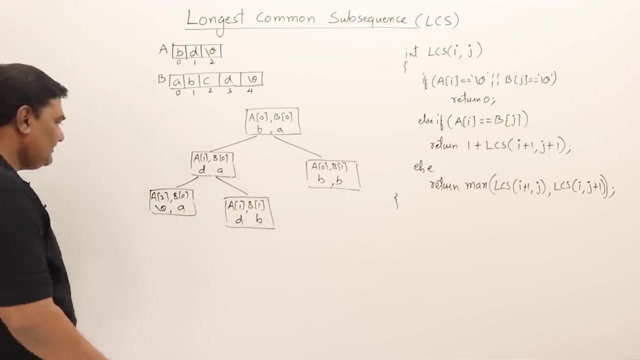 more call. so this is A1 but B. it will move to the next alphabet. So A1 is D only and B is next B1. so this is B. Now, out of these two, the first one should be solved. See, this is slash 0.. So the first condition will be true, and it. 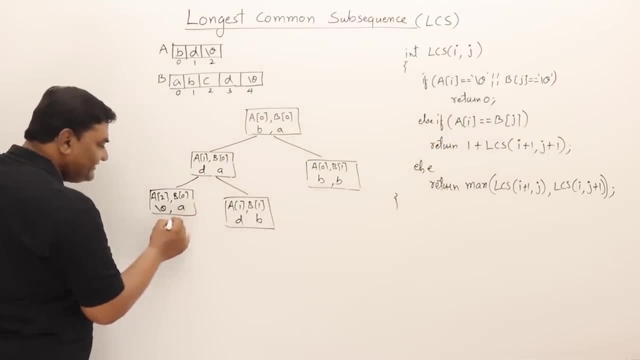 returns 0. So the result of this call is 0. Now this call has to be expanded. So now hope you have understood how it is working so quickly. I will trace the other nodes also. Both are not same so it will go into this part. So first call A will move to the next. 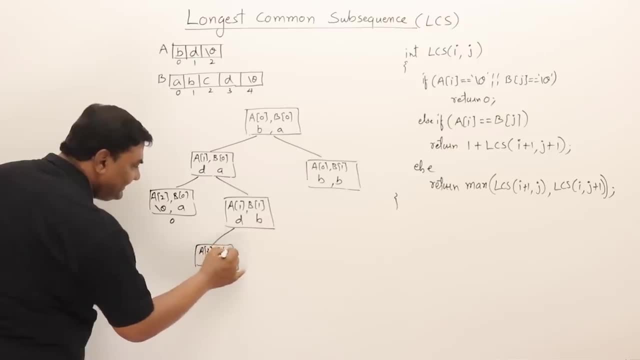 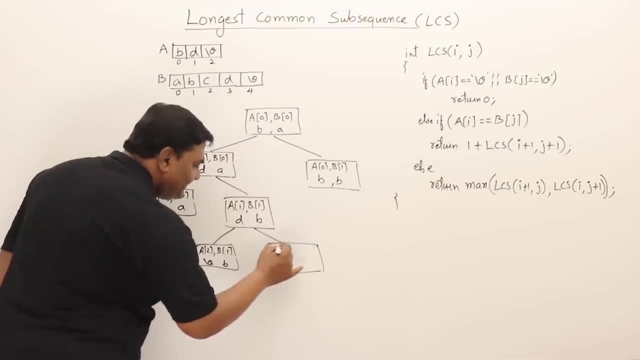 alphabet. so this will be A2 and B remains at 1 only. So this will be slash 0 and that remains B only. And on this side A will remain there only. that is A1, but B1 is 0.. So this will move to the next alphabet. so this a remains a d only, but b becomes 2, that is c. so this call. 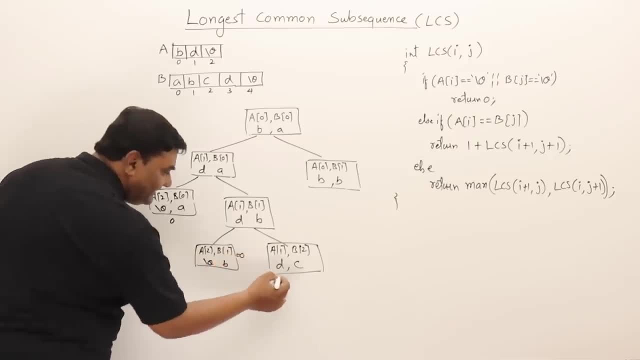 will be finished first. so, but this is slash 0, so the answer is 0. then on this side, again two calls. so this is a will be on 2, b also on 2, so this is slash 0 and this is c only, and on this side. 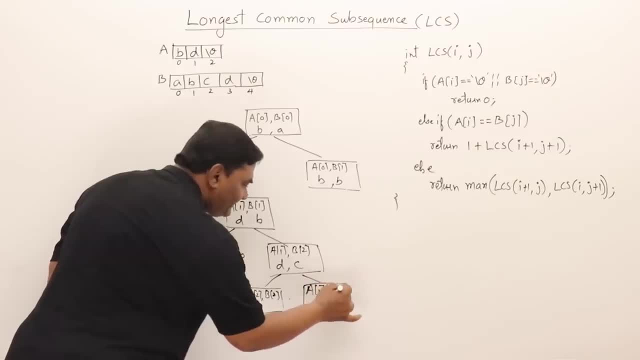 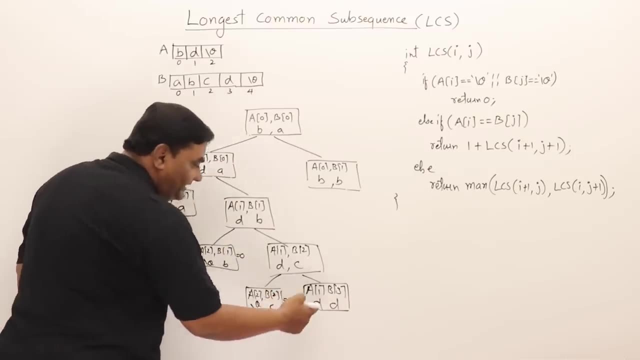 so here it is a 1 only and b becomes 3, and a 1 is a d only, b 3 is what a d? so here the answer is 0, but here they are matching, so it will enter into the second condition. so when the second 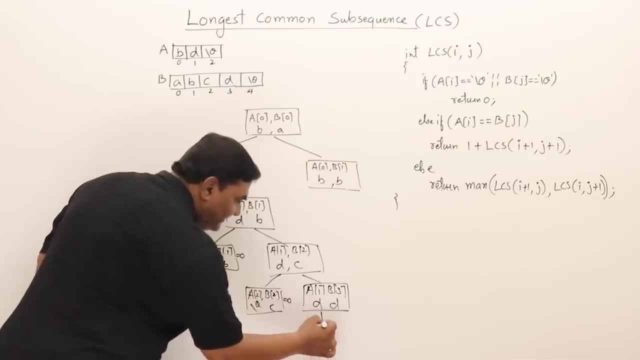 condition. it says that 1 plus and the next call will be: a will also move to next and b will also move to 4. and this both are slash 0 and slash 0, so the result of this is 0. now till, here we got. 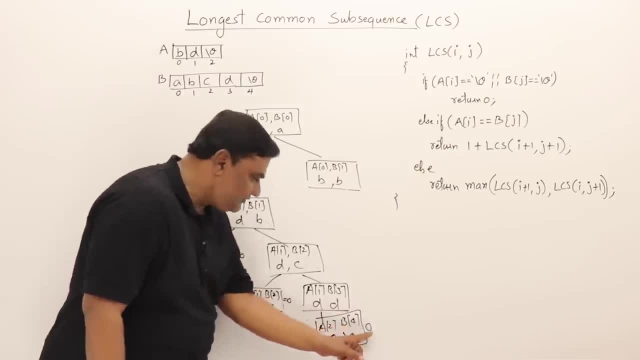 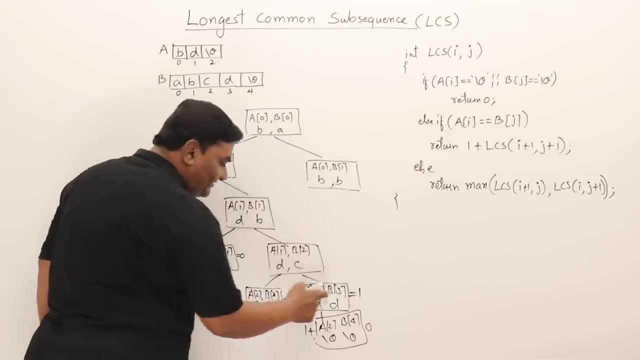 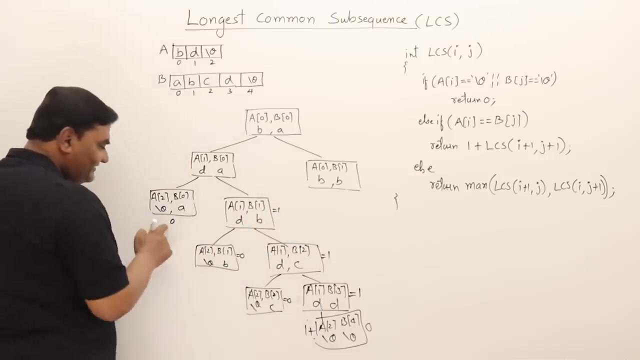 the answer. now it will come back, return back. 1 plus 0 is 1, so the result of this is 1. and what was the result of this? 0, 0 and 1 maximum is what 1, 0 and 1 maximum is 1. now it will start returning 0. this. 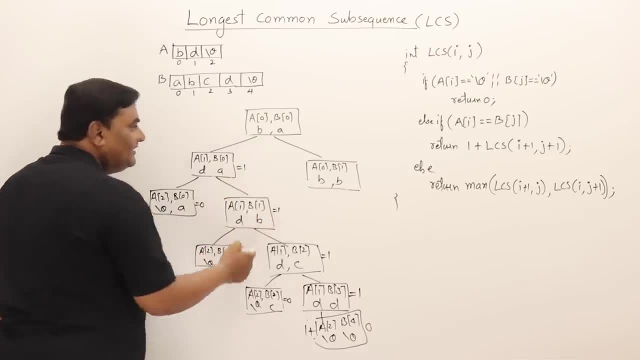 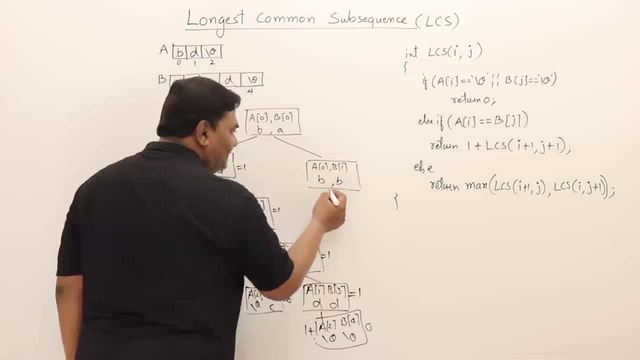 was 0, if you remember. 0 and 1 is 1. now this one is not yet solved, so still, we have to continue with that one. so let us see what will happen. are they matching? yes, both are matching, so it will enter into this condition: 1 plus what is the next a will also move to the next alphabet. 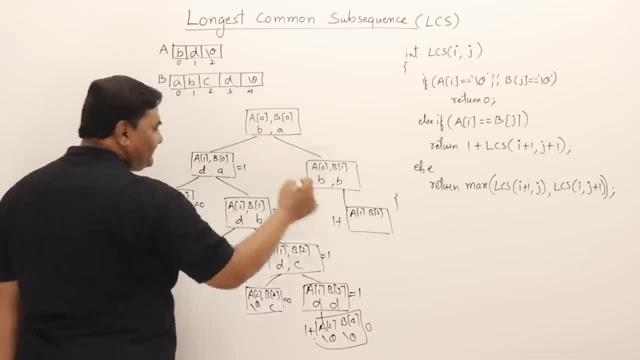 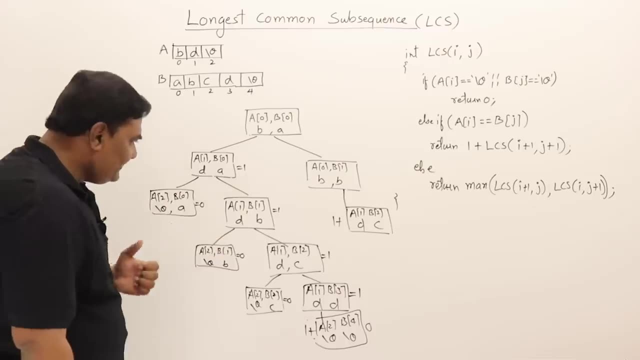 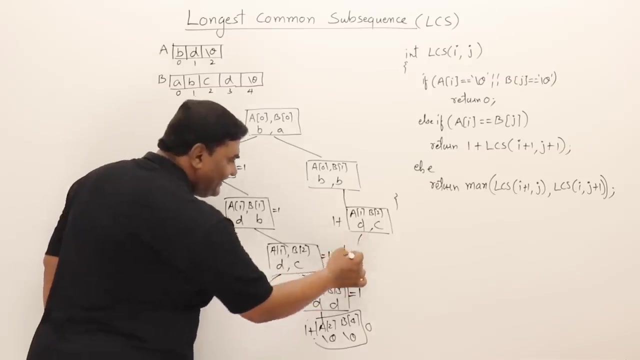 b will also do the next alphabet. so a 1 is what a d and b 2 is what c. so this is dc. now, if you see, this is matching with this one. but this is recursion. this will continue, so i will not explain. simply i will write on what are the nodes you will get here, so just the font size is little. 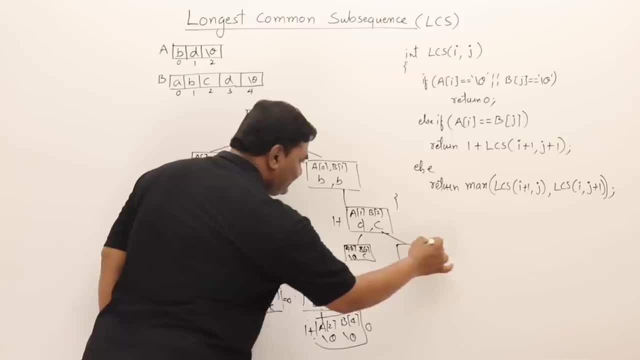 bit reduced now because of the space and this side it is a 1 and b 3 and this is dd, and here it is 1 plus a 2 and b 4, and these are slash 0, slash 0. this is 0 result. 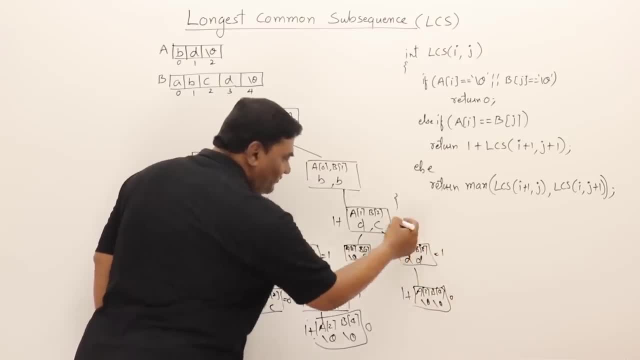 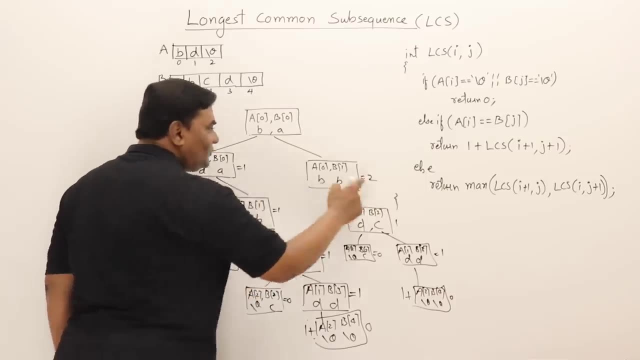 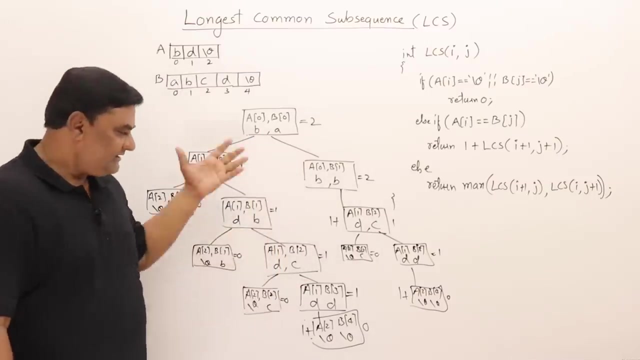 is 1, this is 0. result is maximum is 1, then 1 plus 1, 2. so 1 plus 1 and 2, maximum is 2. so yes, that's the answer. so finally, the answer is 2 and this is a recursive algorithm and it's a tracing. 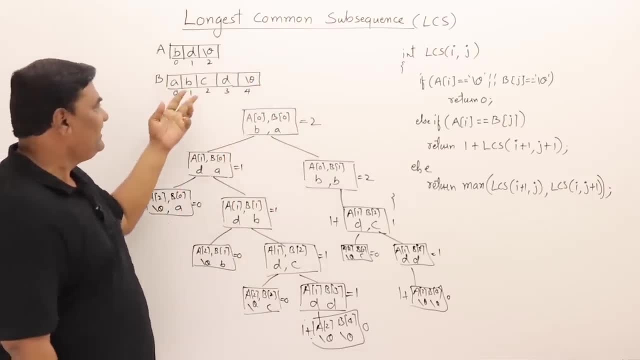 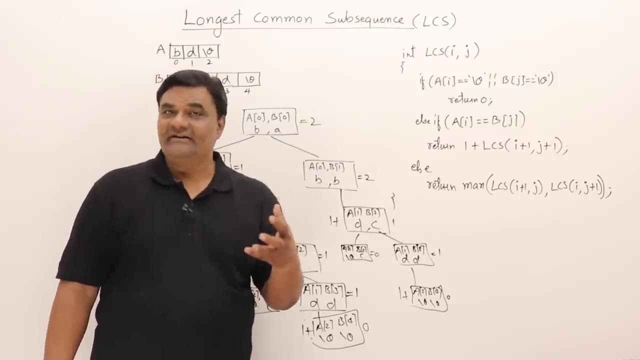 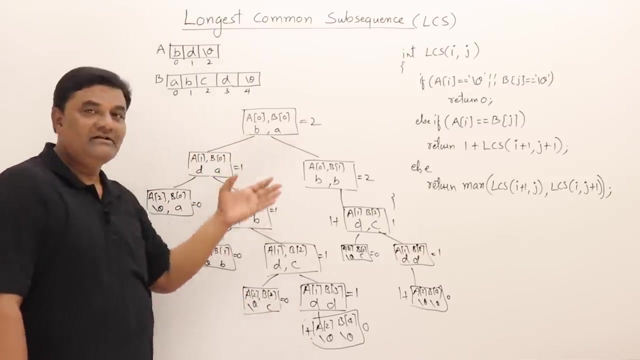 tree for this algorithm upon this example, see for just two, three alphabets only. a tree is such a huge tree so it's exponential time taking algorithm and from where it is starting, from top, that is first alphabets onward. it has started from top, then answers it is getting while returning. but 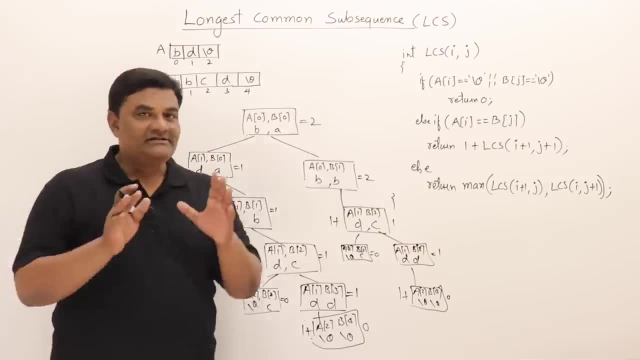 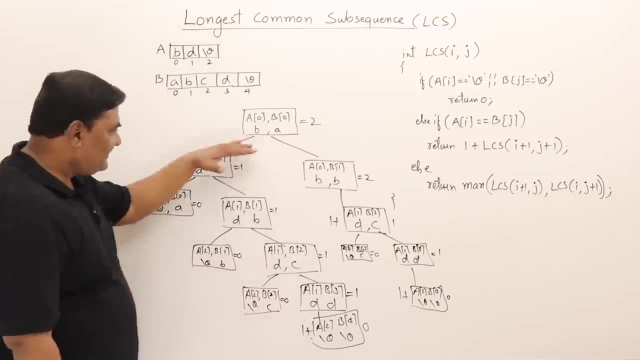 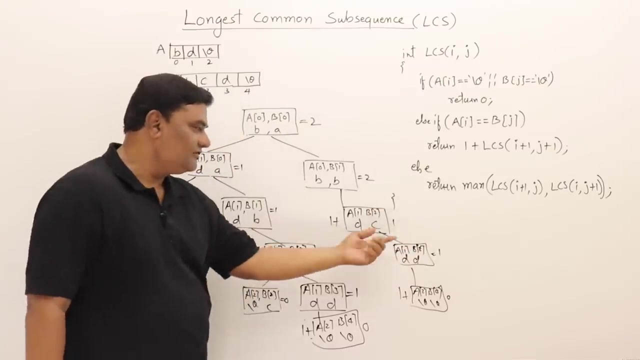 it has started from top. so this is top down approach. now let us understand. what was the purpose of showing you this one? see, the purpose is here. there is an overlapping problem already this side. when we solved, we got d and c and the answer was 1. so here also the same thing we are getting in this branch also. 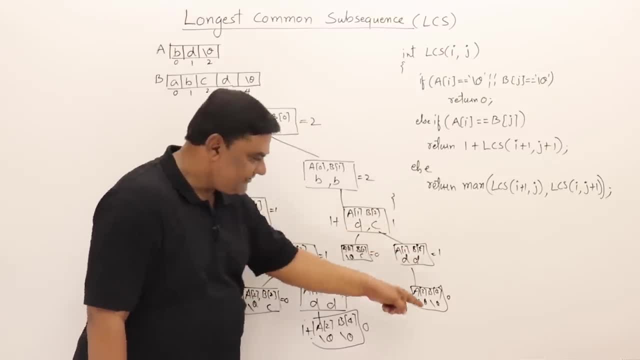 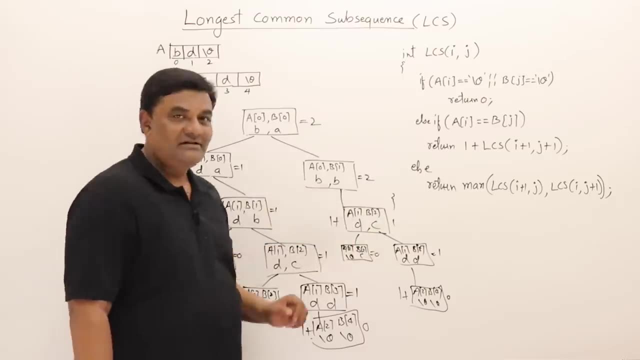 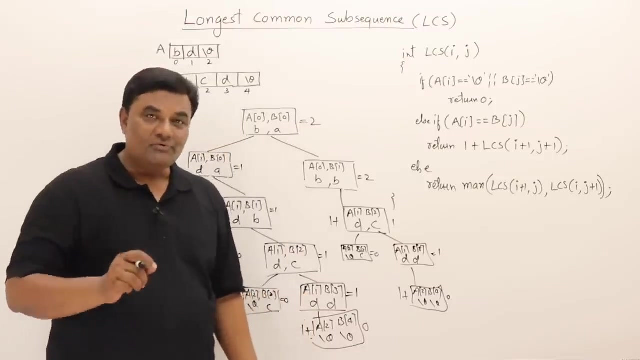 so it means: shall we call these function calls or algorithms? again, there is no need of recursive call if you can remember this answer, so where you can store it somewhere. so if you are storing the results of recursion then it is called as memoization. so to improve recursion you can. 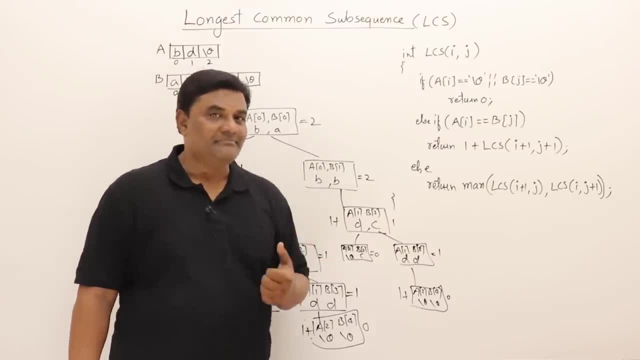 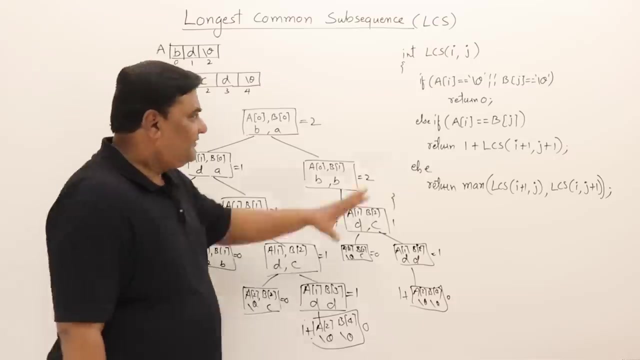 take the help of memoization and you can reduce its time. in my example, only a piece of tree is overlapping, but if your problem is a big, then lot of branches may be overlapping. so let us finally understand how memoization can make this algorithm faster. i will not change the code, just i will prepare a table and show you how. 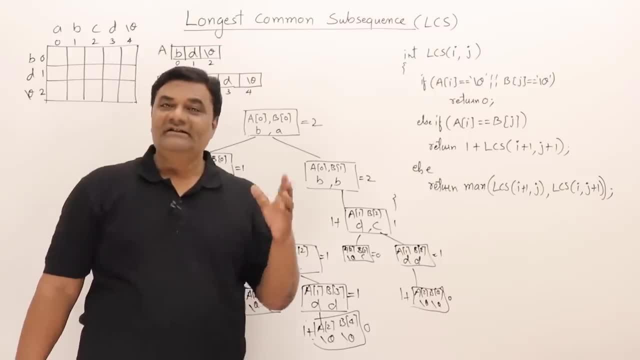 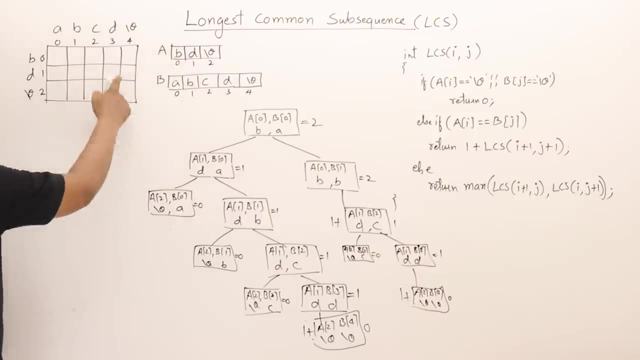 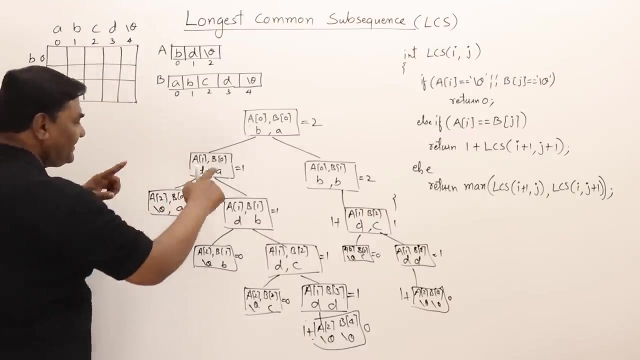 memoization can help this one. so i have taken a table for these two strings for memoization. see, the rows are representing the first string, a and the columns are representing string b, and I have taken the indices from zero onwards. Now let us see how this algorithm can. 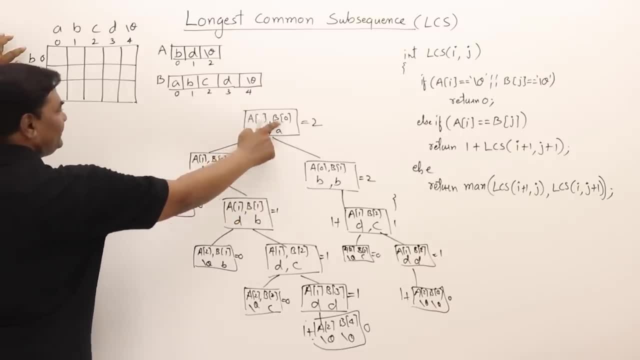 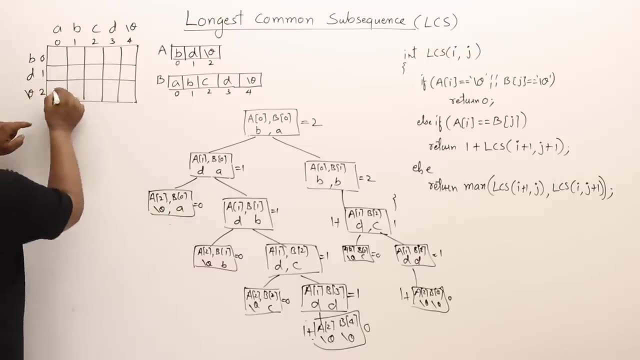 utilize this table to work faster. So first we will start from 0: 0, then 1: 0, then 2: 1.. So first 2: 0.. So the first value that we get is for 2: 0 and that is 0. Then it will move on to this, then. 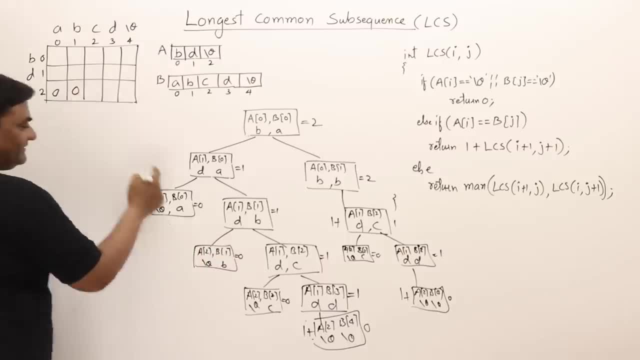 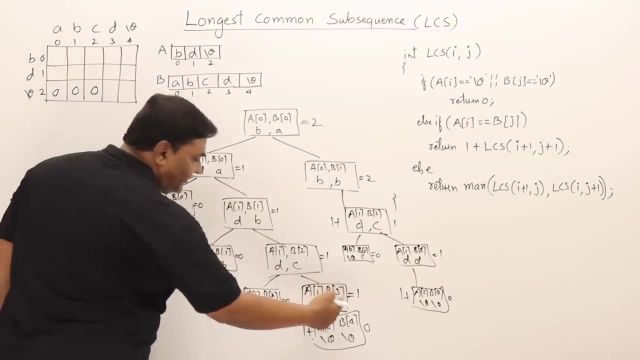 this one Second value we get is 2- 1 and the answer is 0. Then next it will make a call to this and call to this, So we get the answer for this one that is 0. 2 to 2 is 0. Then it will make a call. 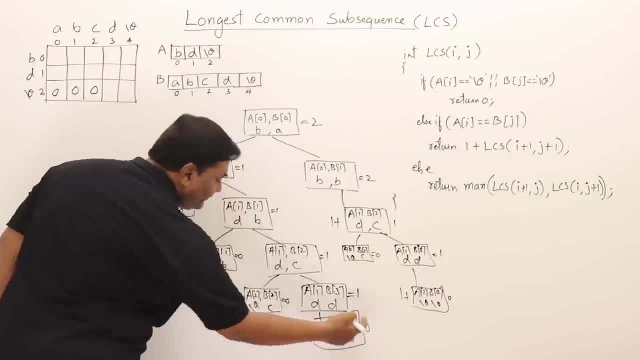 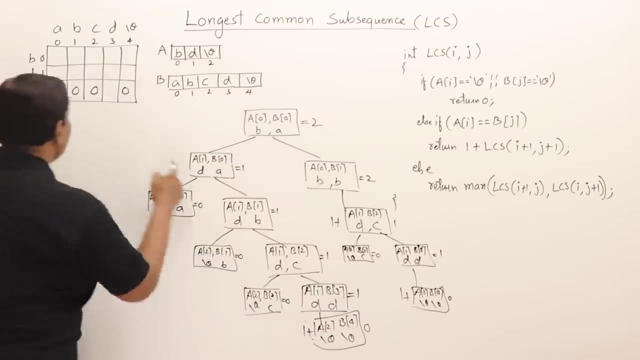 here and this call So for this also. we get the first value, that is, 2 comma 4 is 0. Then it return back and the result of this one is 1.. 1 to 3 is 1.. So it is 1 to 3 is 1.. Return back and 1 comma 2. 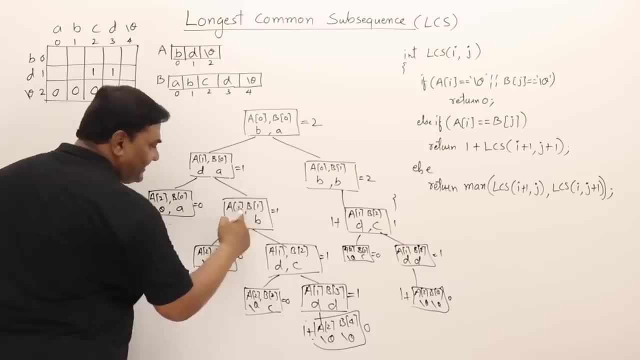 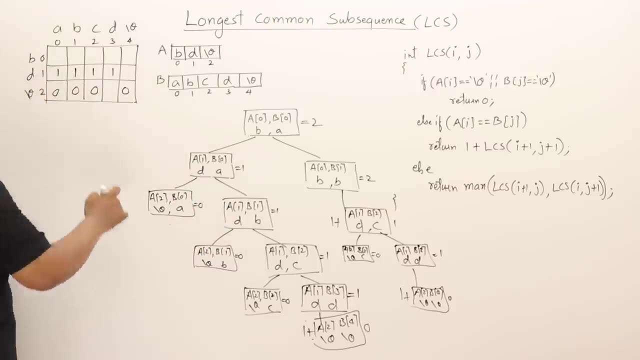 is 1.. So the answer is: 1 comma 2 is 1, and again it turns back, So 1 comma 1 is also 1.. 1 comma 1 is 1.. Then returns back, So 1 comma 0 is 1.. 1 comma 0 is 1.. See, this is top down, but the table is. 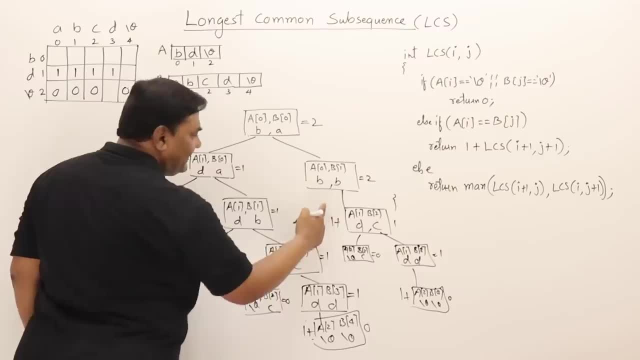 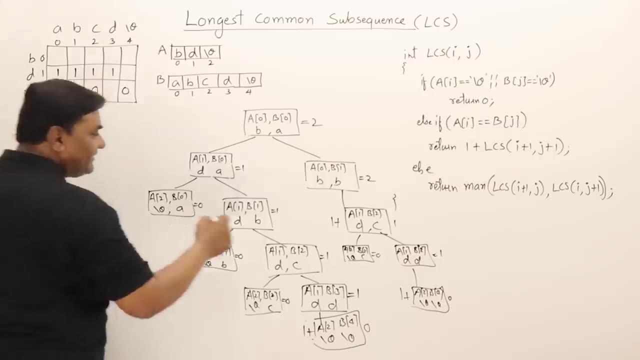 getting filled from bottom towards up. Now, this side it will come and this is the value that we get. See, but this 1 comma 2 already we know the answer. 1 comma 2. yes, we know the answer, So no need to make these calls. So that's how it will. 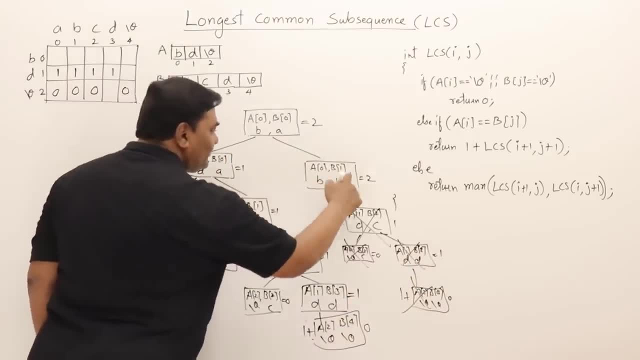 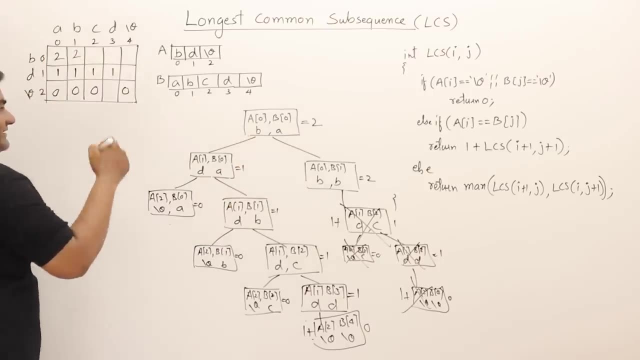 save the time. Then directly it can get the answer for 0 comma 1, that is 2.. Then finally, 0 comma 0 is 2.. That's it. So we got the answer. See the value of this 1 comma 2 was already there in the table. 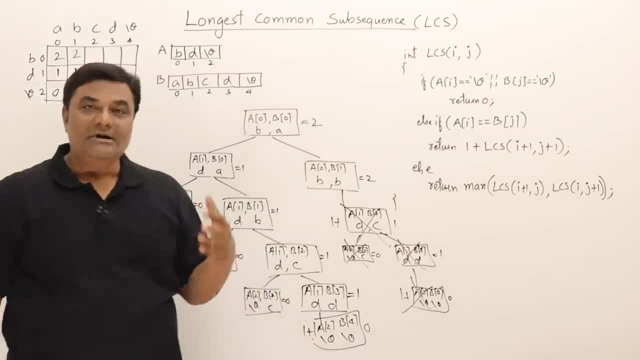 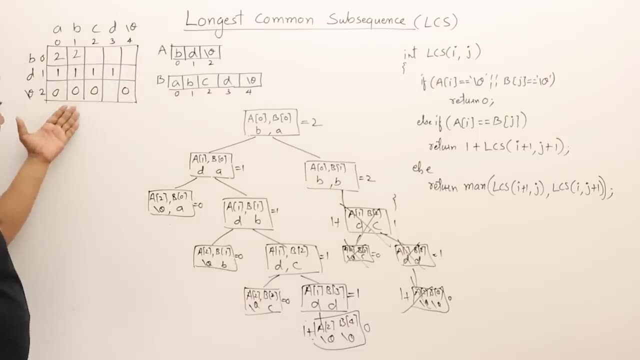 So we did not make these function calls. So memoization can reduce the number of function calls. So total how many calls were made that are there, depending on the number of elements in a table. So that depends on this one. So what is the size of this one? So if this is m and this is n, so the time is order of m. 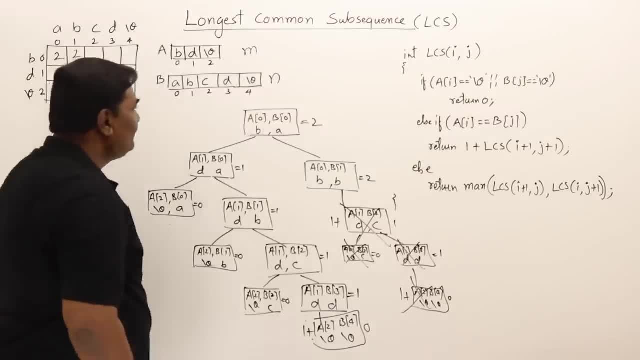 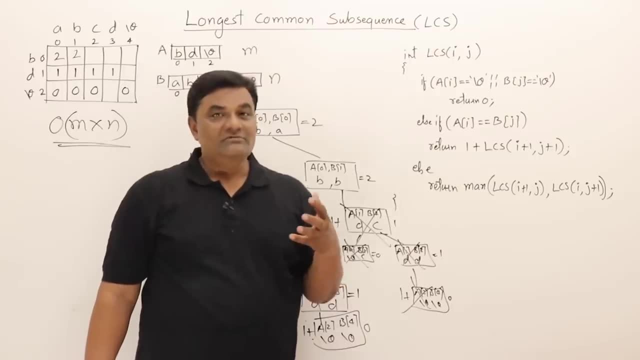 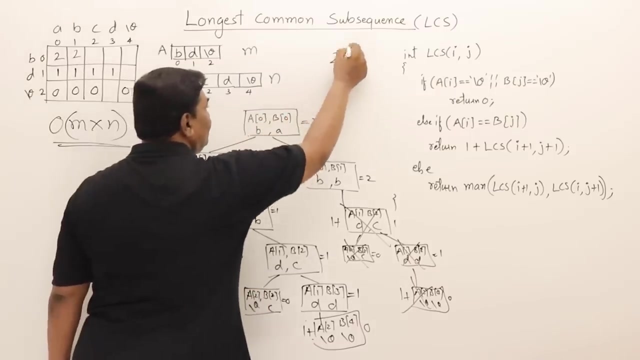 cross n. So the memoization is taking order of m cross n time for solving a recursive algorithm. That's all. So this was top down approach and we have taken the help of memoization to reduce the time complexity from 2 power n to m cross n. 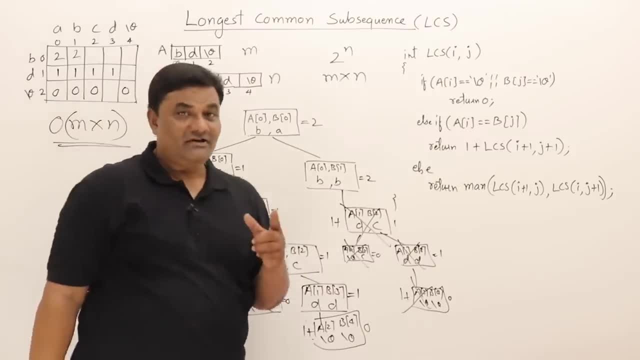 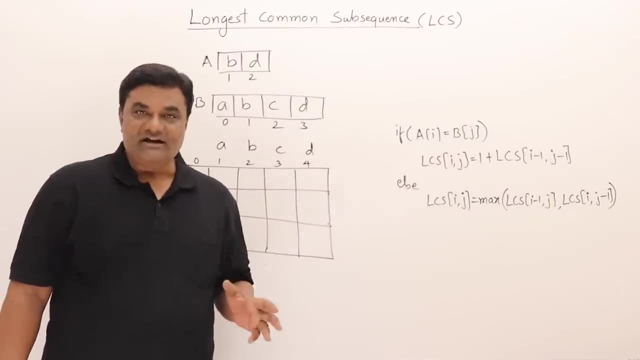 Now, finally, we'll see an algorithm for dynamic programming For the same example. I will solve it using dynamic programming. So let us solve our problem using dynamic programming. So you know that dynamic programming follows bottom up approach. So in the previous example, when we solve it using recursion, the table was getting filled from bottom towards up, but the method was top down. 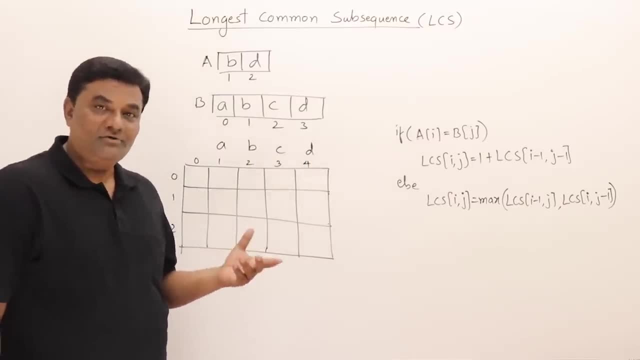 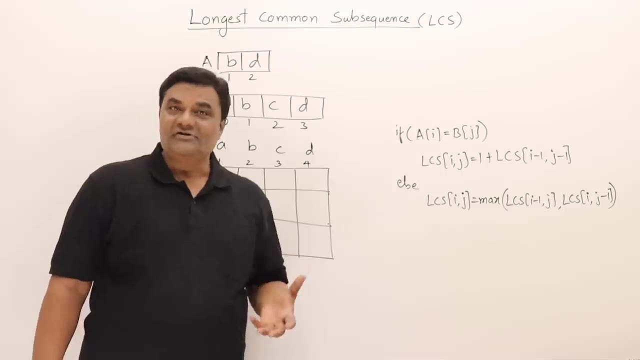 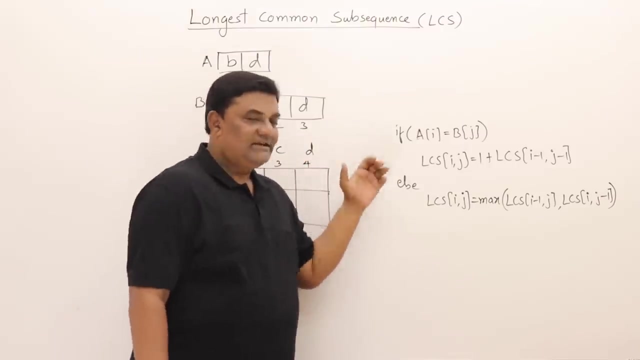 but now, dynamic programming follows bottom-up approach, but the table will fill from top to down. so it's not based on the filling of a table, it's based on the approach for solving a problem. so let us see how to solve using dynamic programming. see, this is the algorithm for dynamic programming, if there is a. 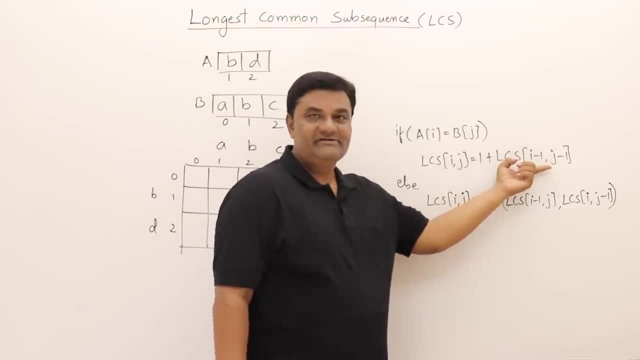 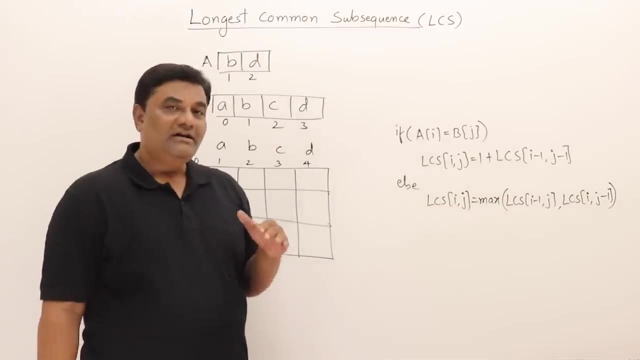 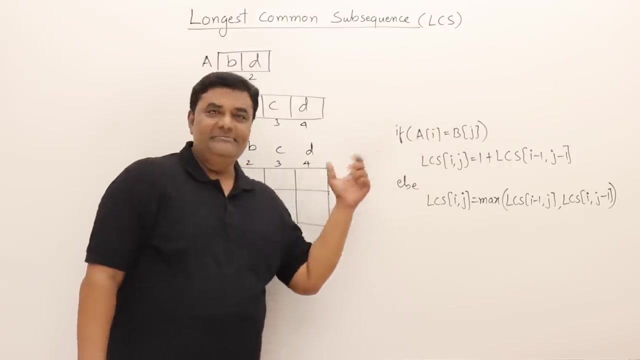 match, then you add one and take the value from the previous diagonal element. if there is no match, then take the maximum out of either previous row element or previous column element for a particular cell. so let us see what does it mean by solving the problem. I have taken the same example, but here you can. 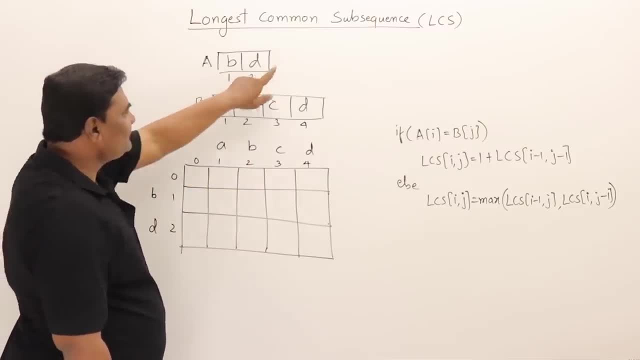 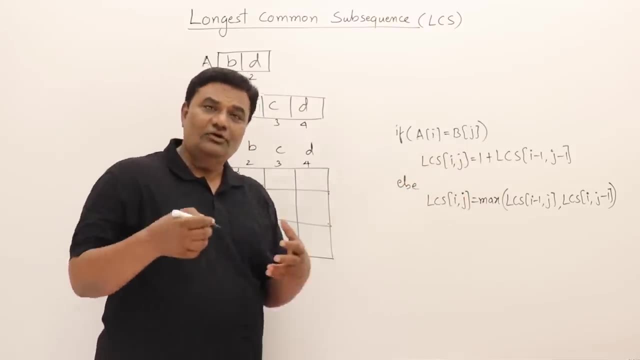 see the indices. for this one, I have started mix from one onwards and there is no slash 0 because the algorithm, the way it is written it, is not involving slash 0 and starting indices from 1 onwards. if you want to modify it, you can modify it and include slash 0 also. start index from 0 also, but commonly found. 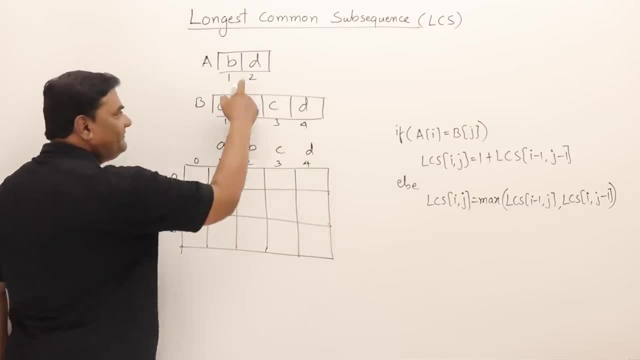 algorithm that works from index 1 onwards. so I have taken index from 1 and 2. this is 1, 2, 3, 4. then here we are still using index 0 because we want the initial values here that to be filled with a 0. so that will help the algorithm. 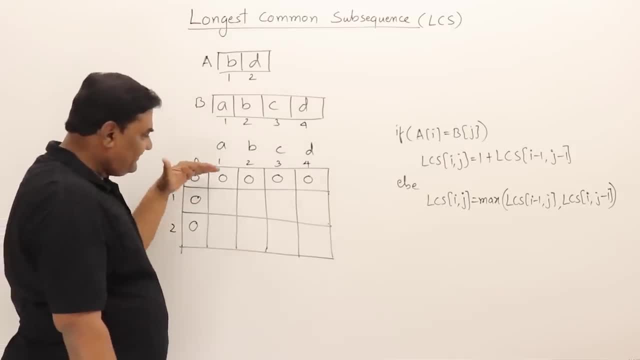 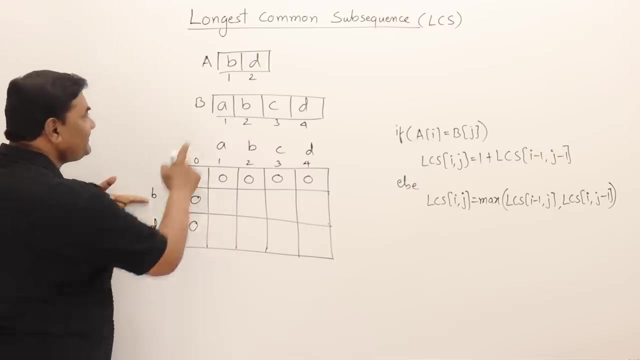 to start, from this point onwards, table filling from top towards bottom, but the algorithm working is bottom-up. let us see how to fill this. it's very easy and very simple. see, I have to fill all the elements in this row and this row. so, row by row, I have to fill the element. so what I have to do is- see this is string. 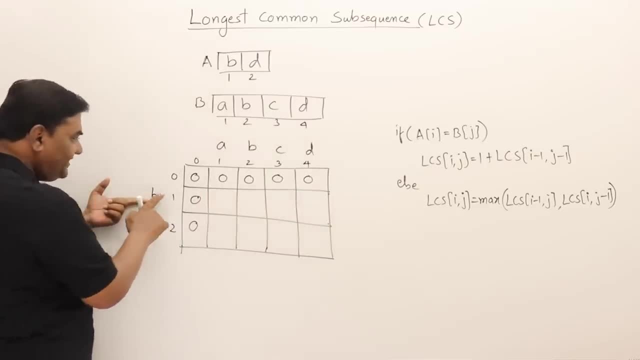 representing a. this is representing B, so check if B is found anywhere. so first start with this one. is it same as B? no, they are not matching, so take the maximum of these two. this condition, so that is 0. 0 is 0. only then B is matching with this one. yes, matching. 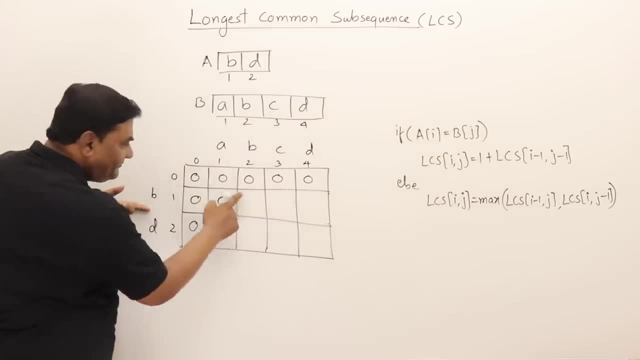 so the first one, 1 plus a diagonal element, 1 plus this diagonal element, 0 plus 1. 1 then is a, C and B are matching. B and C they are not matching, so else part maximum of these: 2. this is 1. this is previous column, this is previous role. 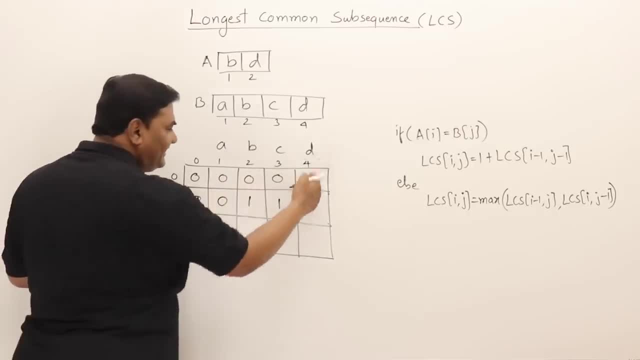 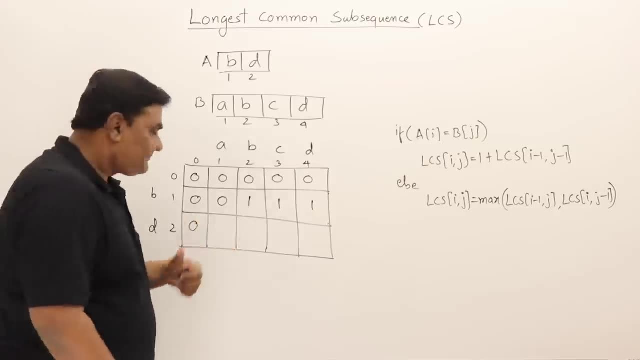 for this particular cell. so this is one only. B and D. they are not matching. so. previous column, a previous row here, maximum notice: that is 1, only now. next row: d à not matching maximum of these 2. D and D not matching maximum of these 2. 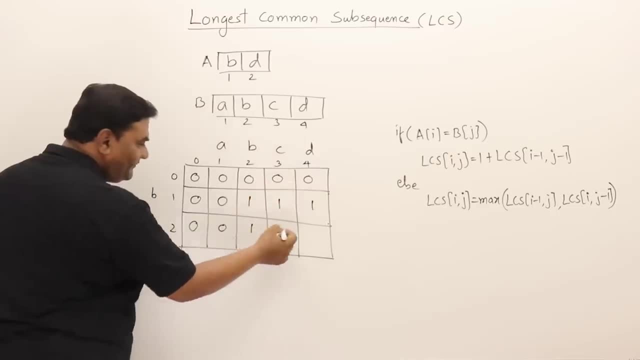 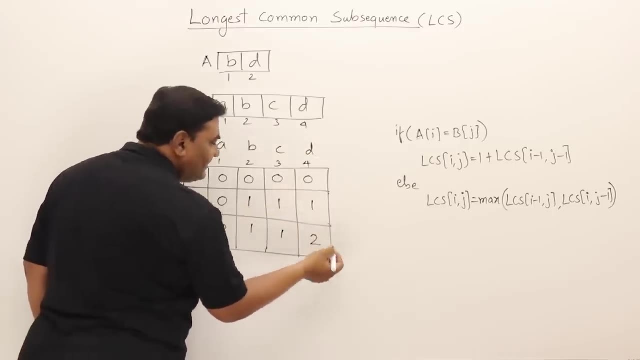 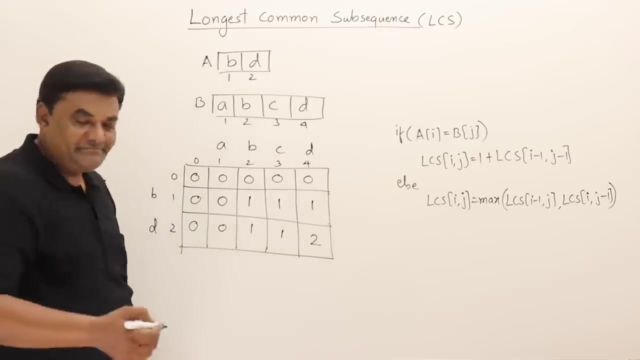 1 B and C not matching maximum of these. 2: 1 D and D. they are matching. so diagonal plus one, one plus one two. that's it. so the size of the longest common subsequence is two. but what is the longest subsequence? so let us trace back two. we got this two by adding one to. 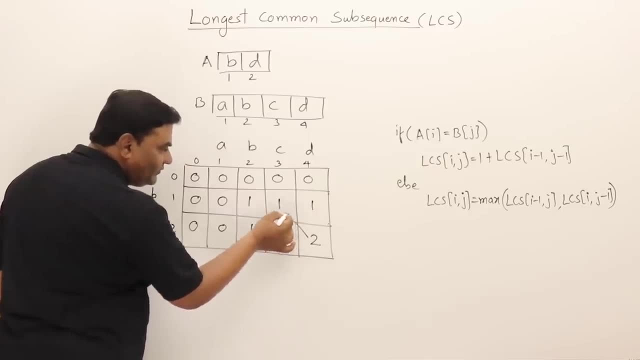 this because both of these are one one, so go diagonal. and then this one: we got it from here, yes, this one, we got it by adding one to this one, because none of them is one, you see, so this is coming from here, right, this one, because already this was one, so we said that we have taken it. 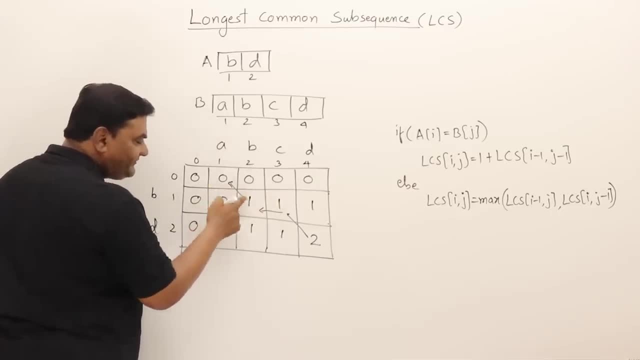 from here. but for this both of these are zero. zero it means we got it by adding one to this now, where we have gone in diagonal at this place. so what was the alphabet? d? and the other place where we have gone diagonal, this was b, so this is bd, so bd is the sequence. 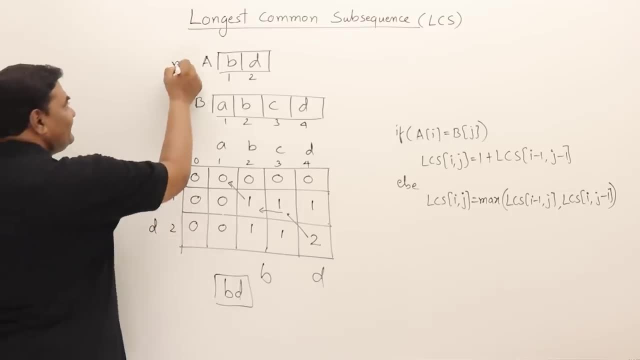 see how much is the time taken by filling this table. this is m number of alphabets. this is m number of alphabets. this is a Murdawartha, declared the whole thing. so before, only bdt besides bdt. so before only bdt: other alphabets不同. so after only bdt: alphabets ofi, rc, qums. give some remind. 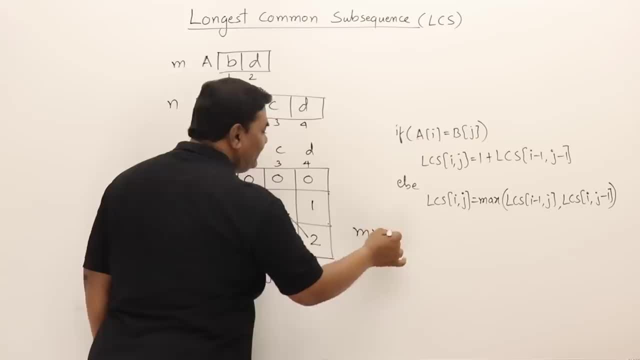 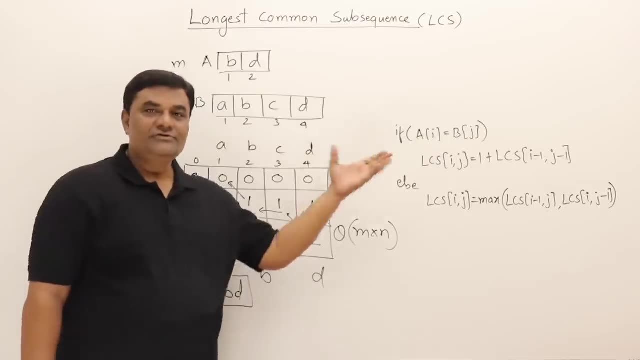 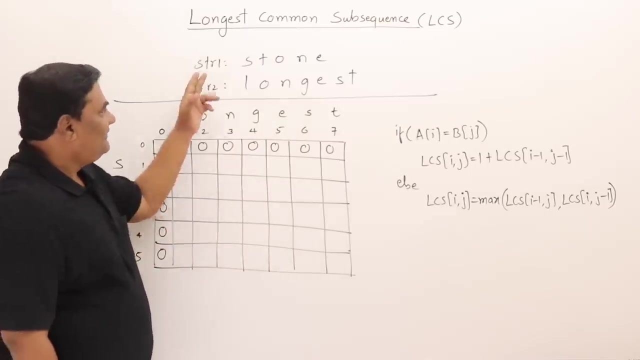 number of alphabets, so total number of cells are m into n, so the time is m cross n. now i will take one more example and show you a simple example and show you how it can be solved using dynamic programming. let us solve this small problem using dynamic programming. i have two strings. one is a. 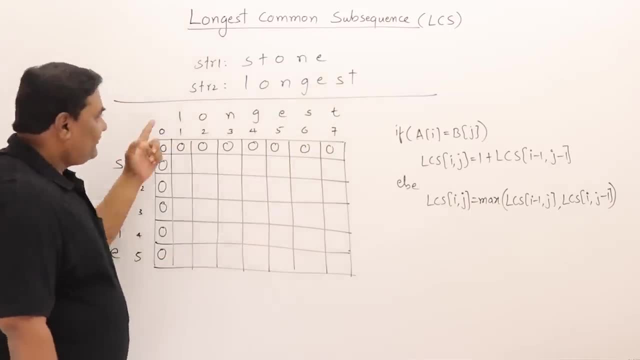 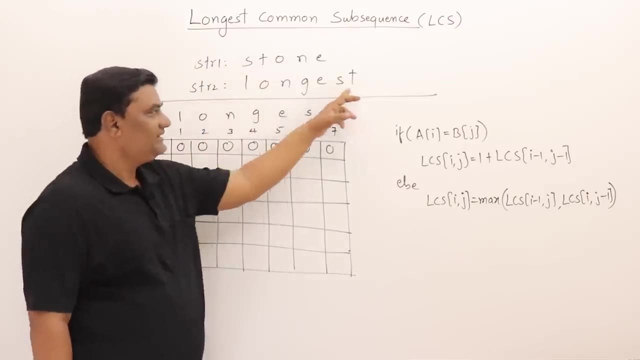 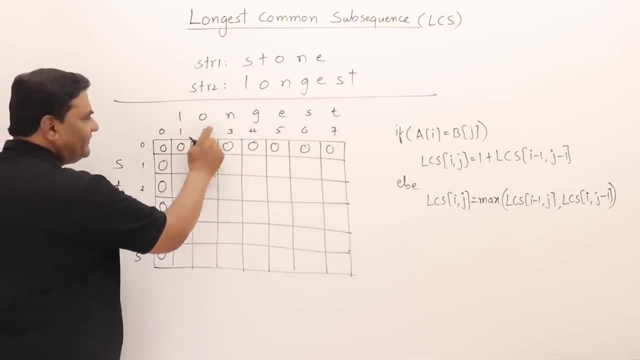 stone and other one is longest, and for that i have prepared a table: rows are equal to the number of alphabets here and the columns are equal to the number of alphabets in longest, and index 0 is reserved for initial values of 0. so i am starting indices from 1 onwards: 1, 2, 3. so these are all the. 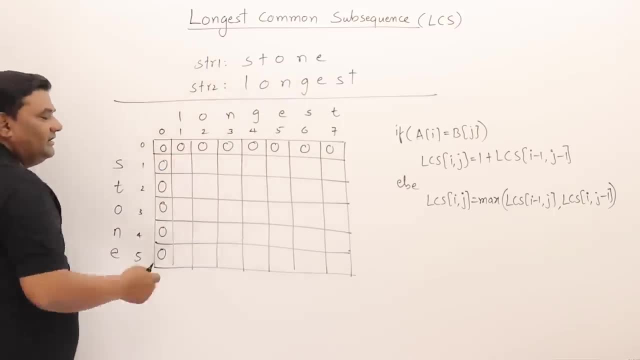 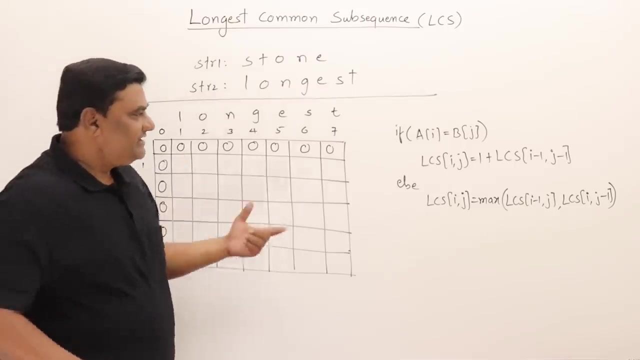 alphabets of longest. these are the alphabets of stone. so let us find out what is the longest common subsequence and as well as what is that subsequence? so for that, we will follow this algorithm and just fill up the values. we will get the answer. so what the algorithm says. well, 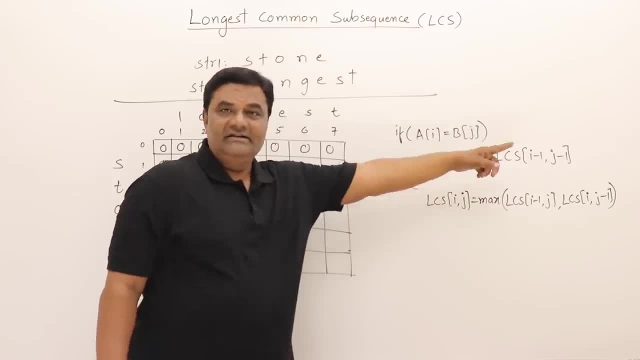 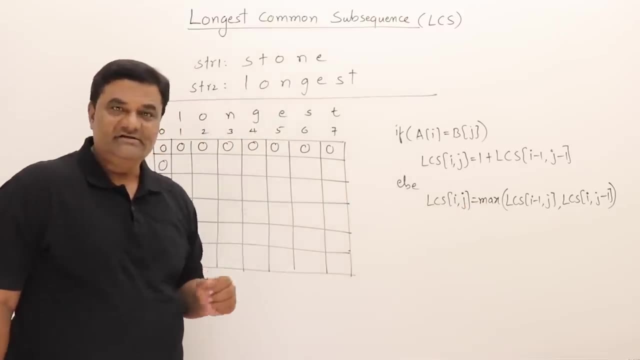 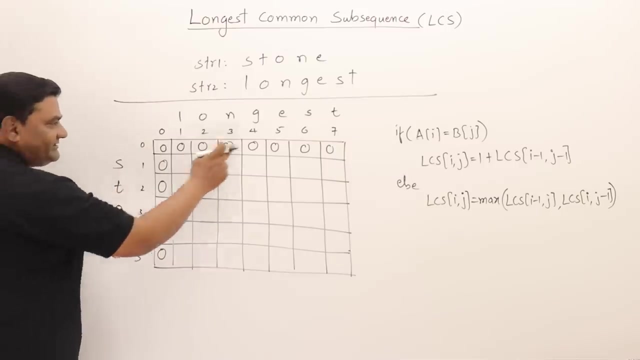 whenever there is a match, take the value plus 1 and take the diagonal value. If there is no match, take the maximum either in the previous row or in previous column for the same cell. So let us follow that. I will show you quickly how this can be filled. First alphabet: let us start already this. 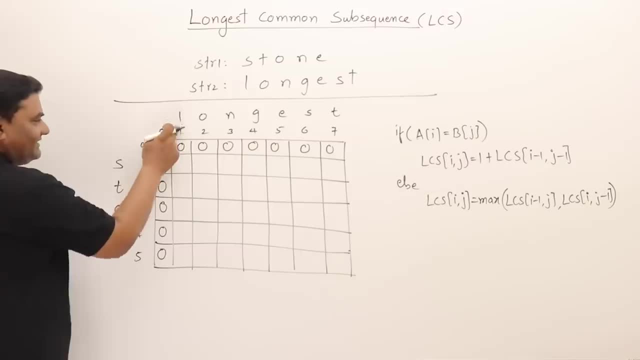 is initialized to 0, so from here I have to start s there is no match with l, so take this value or this value, and that is 0, only s not matching. so 0 or 0. take 0, only this, not matching 0, more not. 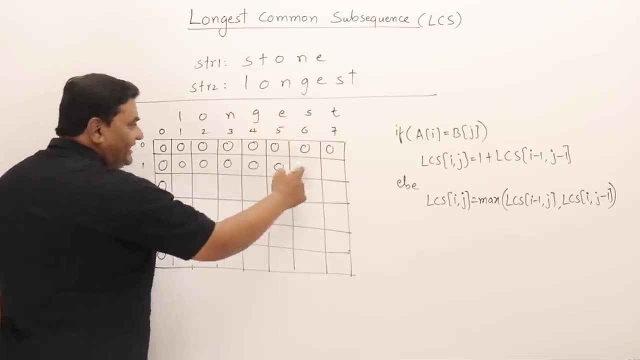 matching 0, 0, s and s are matching, so take the diagonal. add 1 to that. 0 plus 1, 1. the next s and t are not matching, so take anything of this. that is maximum, so I have to take maximum of this now. 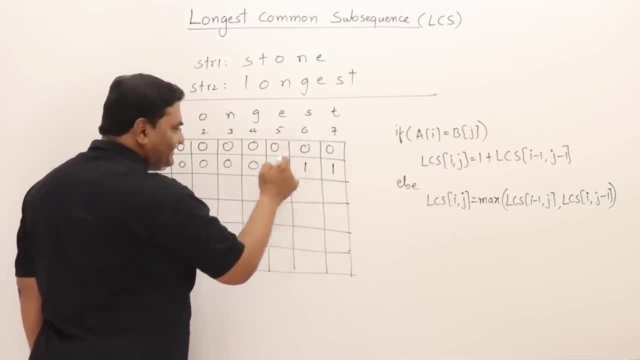 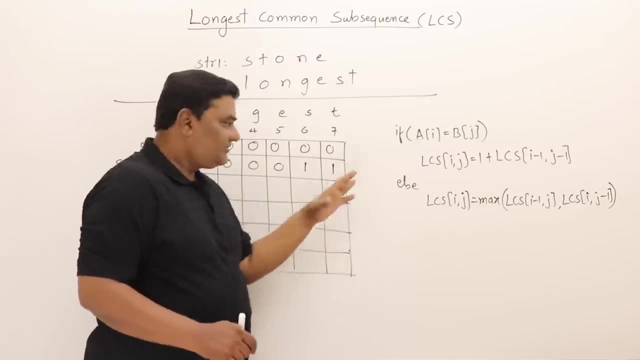 till now it was 0- 0. I was writing 0 only now. this is maximum Now. similarly, we have to do it for t, so you can see that t is matching here at the last. so till there, we will be getting the maximum in the previous row, or. 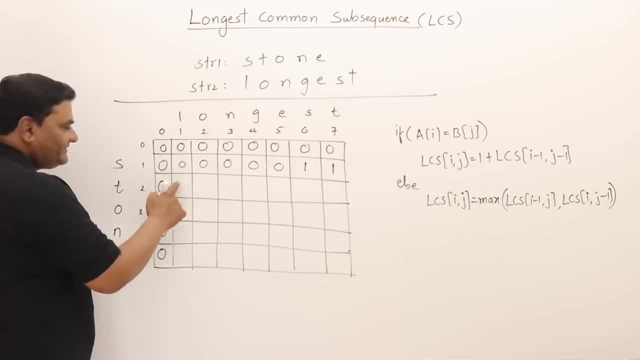 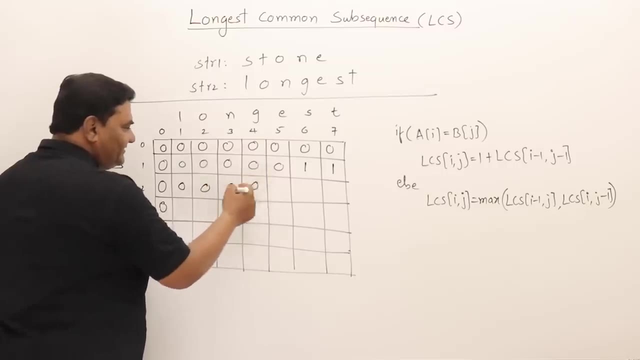 previous column. so this one is 0 and 0, 0, only then 0 and 0, 0, only 0, 0 max is 0. out of these two, maximum is 0. out of these two, maximum is 0. out of these two, maximum is 1 and t is matching there. 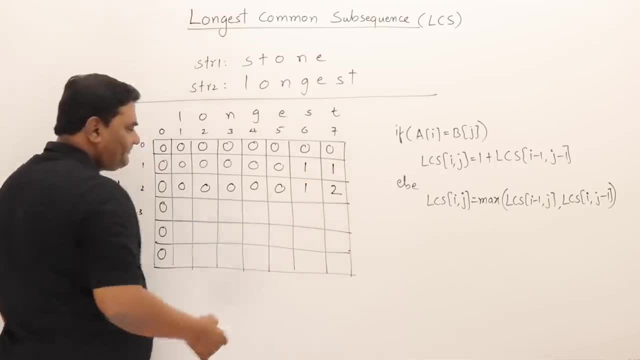 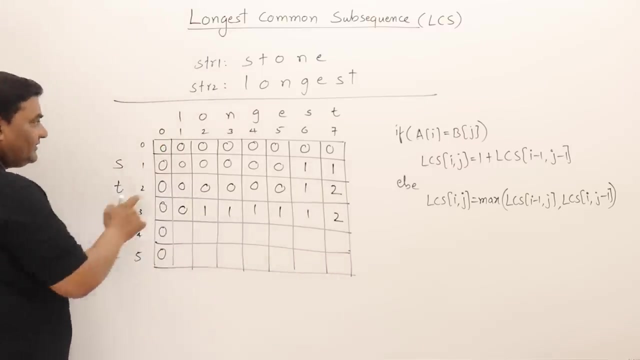 so, from the diagonal, add 1 and take it, so 2. O is matching with this one. so take this value, take the diagonal and add 1. the next is 1, only 1. there is no other match. so simply, I will fill up the value 1, 1, and the maximum of these two is 2. so there is no other O in this string. right? so now n. 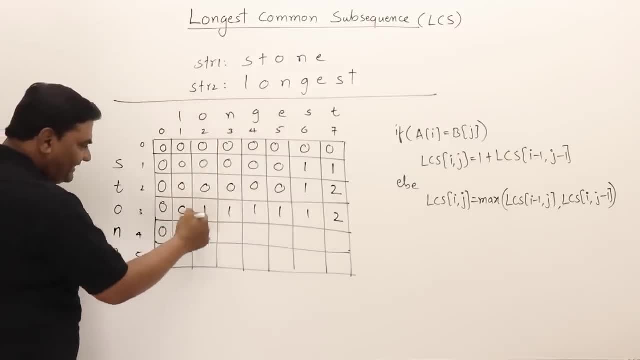 n is matching here. so till there, maximum of these two. maximum of these two, that is 1, but here it is matching. so from the diagonal add 1, 2, see when there is a match, take the diagonal add 1 and write on the value. then after this, there is no match. so we will write on the match. so we will. 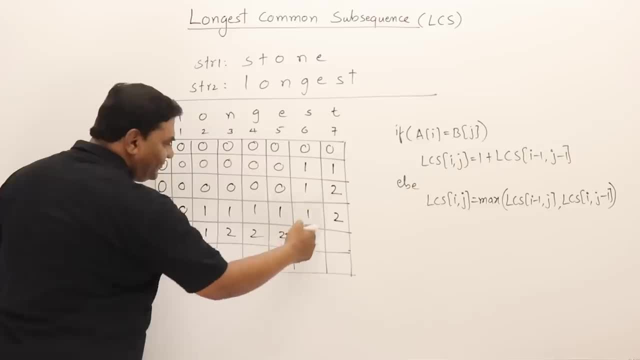 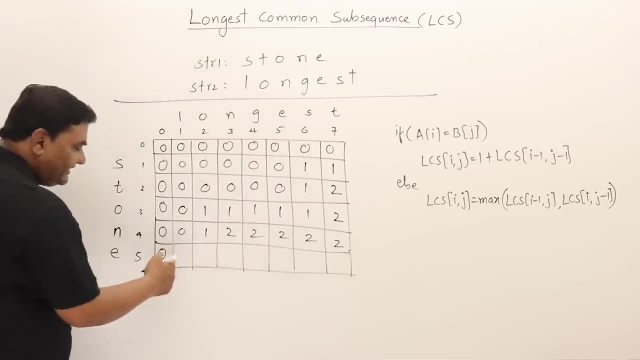 write on the maximum of these two: 2 maximum, 2. maximum of these two: 2. maximum of these two is 2. only then e is matching here. till there I will be writing just maximum. so this is 0 only out of these two. 1. previous column, previous row: 2. previous column, previous row 2. now here e is matching. 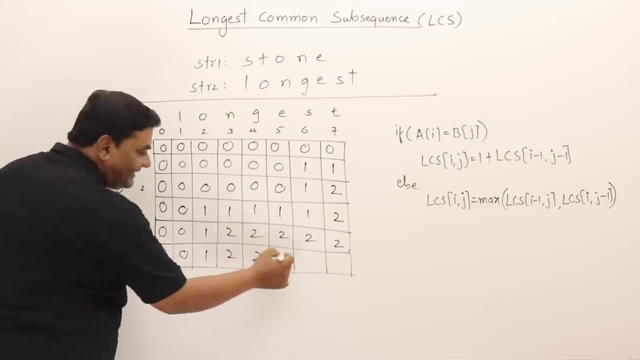 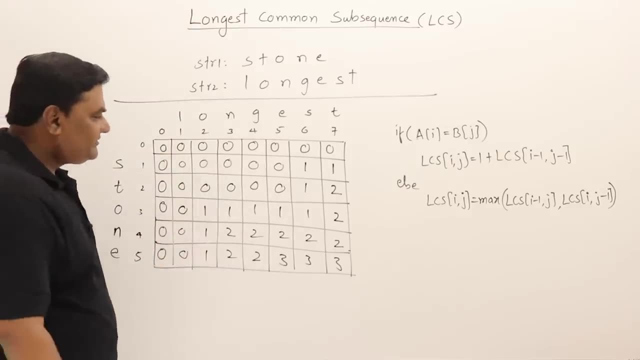 with this one. so take the diagonal, add 1, 3, then after this, 2, 3, 3 maximum. 2, 3, 3, maximum. so the longest common subsequent size is 3. I want to know what are those alphabets? so let us see how to find the alphabets. this 3, we got it from here. that is maximum of these two we 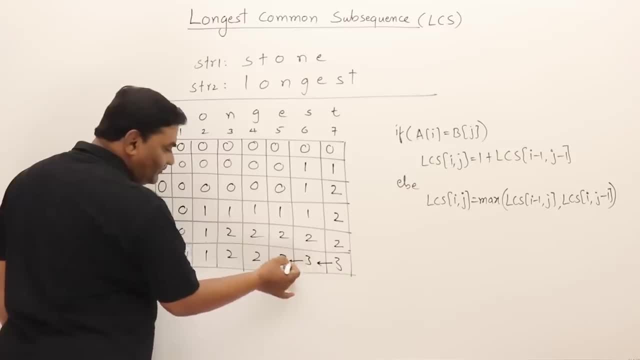 wrote: so go to this one and this 3. we got it from here. go to this one, this 3. before that there was no 3, so it means we got it from this diagonal. so what was the alphabet here? e, then this 2: we got.